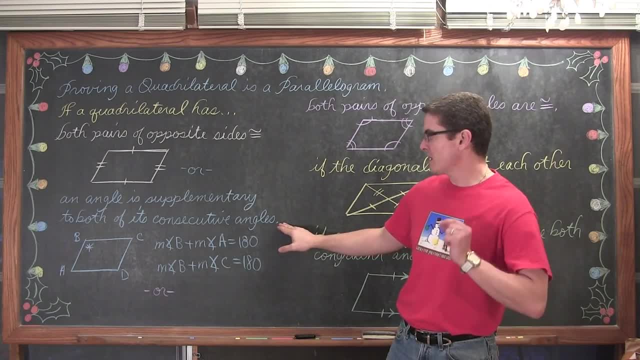 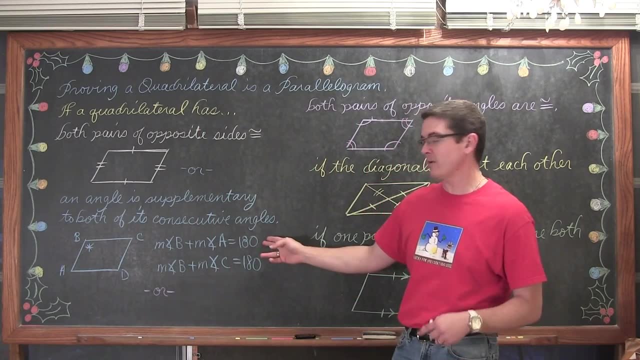 have an angle which is supplementary to both of its consecutive angles. So I just randomly picked B here. If the measure of angle B plus the measure of angle A is supplementary, which means they add up to 180,, complementary is 90, and the measure of angle B plus the measure 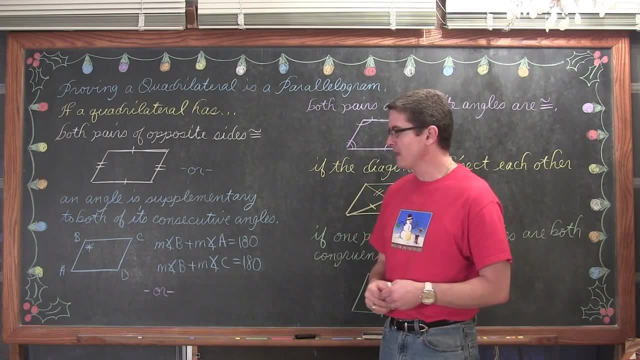 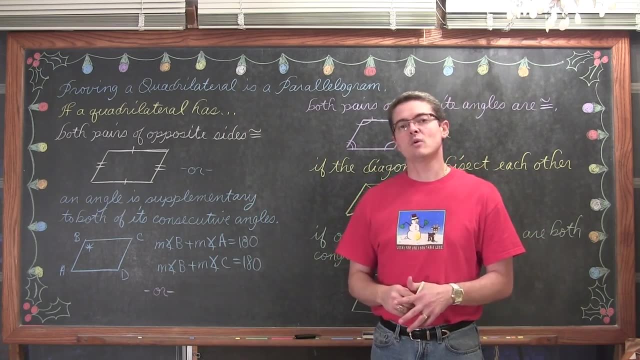 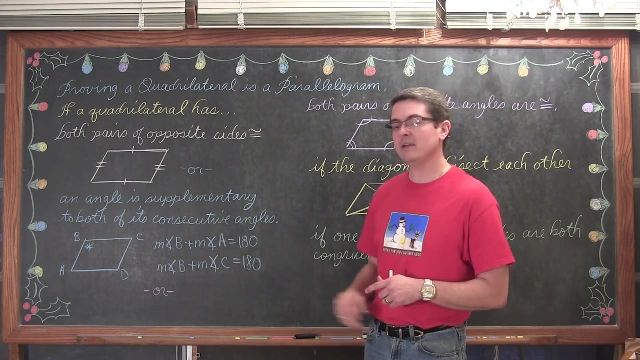 of angle C is also equal to 180 degrees when you add them up then, and that is true for all all of the angles of a parallelogram. but in this quadrilateral, if you just pick any one angle and notice that it is supplementary to its two consecutive angles, then it is. 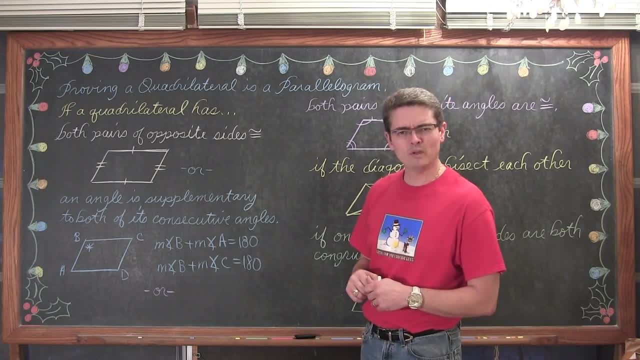 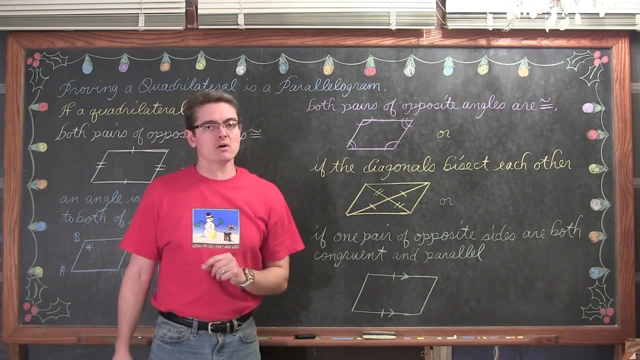 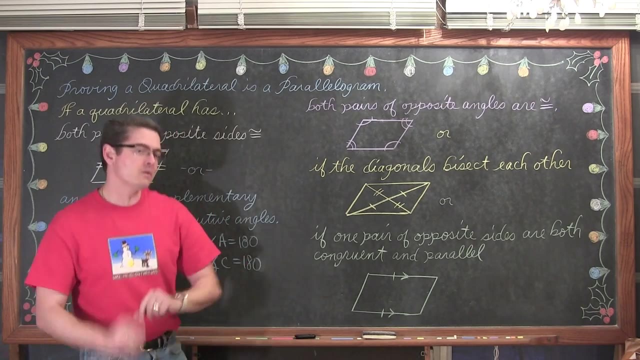 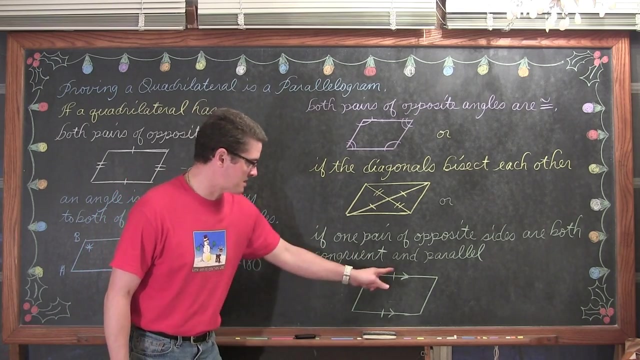 going to be a. hmm, what will it be We have over here? or both pair of opposite angles are congruent, or if the diagonals of this quadrilateral bisect each other, or lateral someday. so, on the last one, if one pair of sides- uh, opposite sides, not consecutive sides. 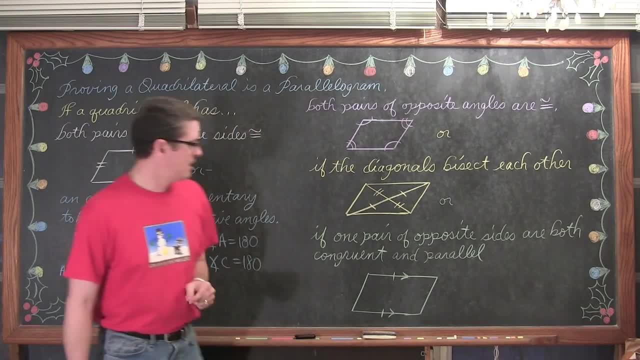 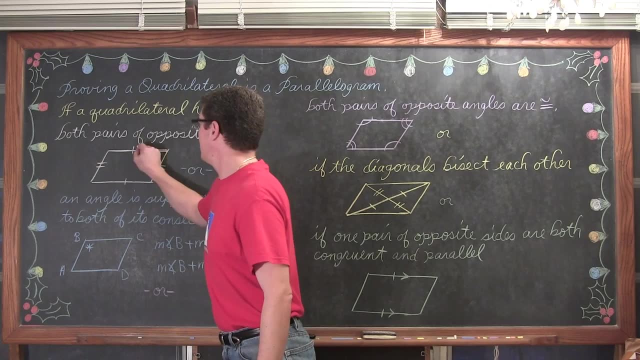 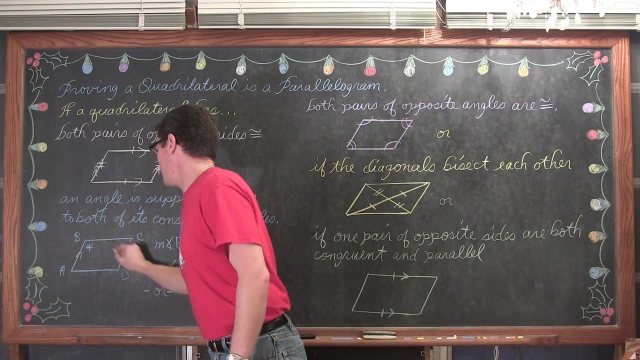 but opposite sides. you have one pair of opposite sides which are both congruent and parallel. if any one of these statements is true, then your quadrilateral is the parallelogram Every single one of these are gonna be. if any one of these statements are true than. 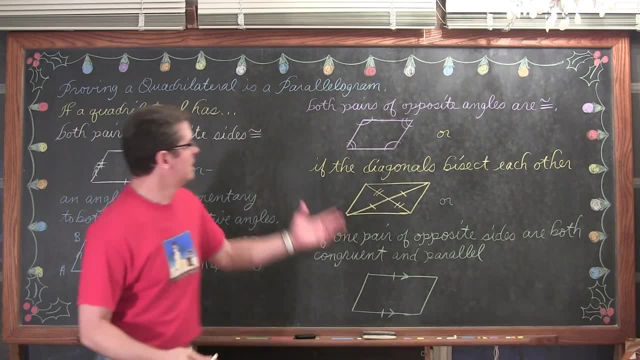 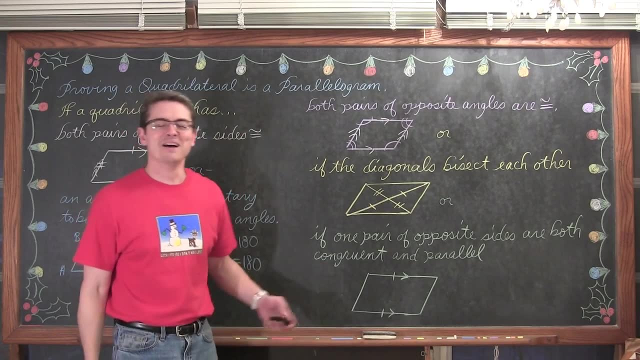 your quadrilateral is a parallelogram. quadrilateral is going to be a parallelogram. I don't think you need to see me do that two more times. Alright, let's get to one of our examples. Solve for x and y to make abcd. 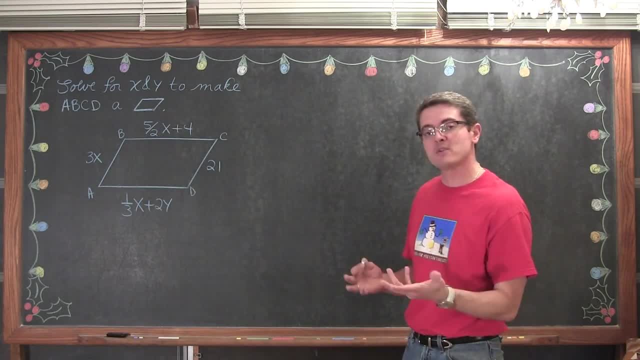 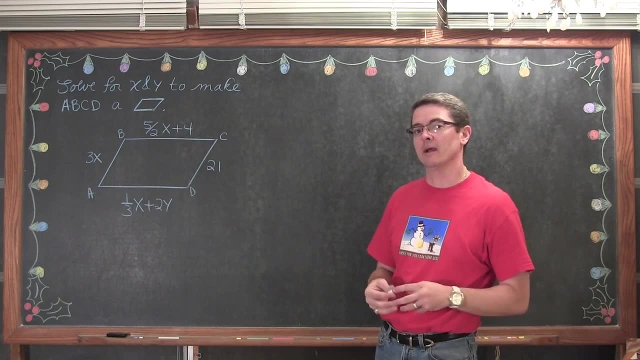 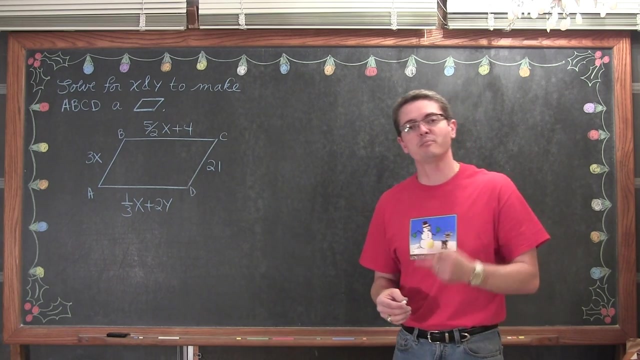 a parallelogram. Well, our expressions are wrapped around the outside of our quadrilateral and I want to ensure that it is a parallelogram. Well, for this to be a parallelogram, one of the theorems that we just erased said that the opposite sides that both pair of opposite. 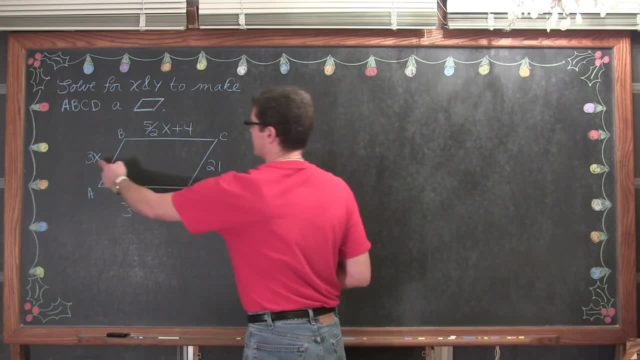 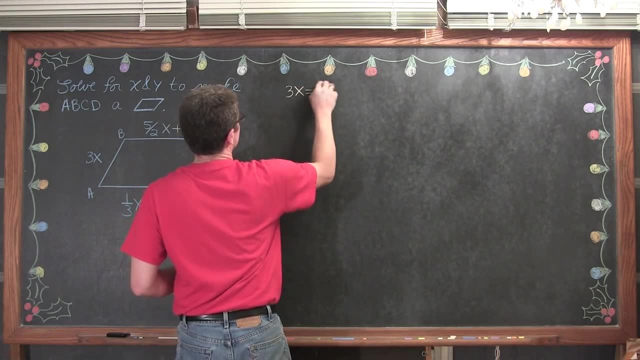 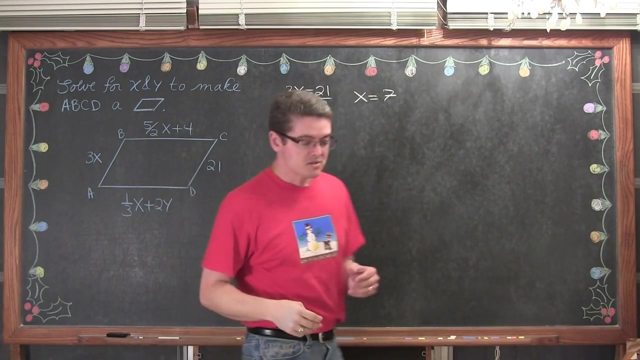 sides are congruent. So if we take our 3x and 21 and set those equal, because that looks pretty simple, we get 3x equals 21.. We are going to divide both sides by 3 and get x is equal to 7.. So x must be 7 to ensure that these two sides, these two opposite sides, 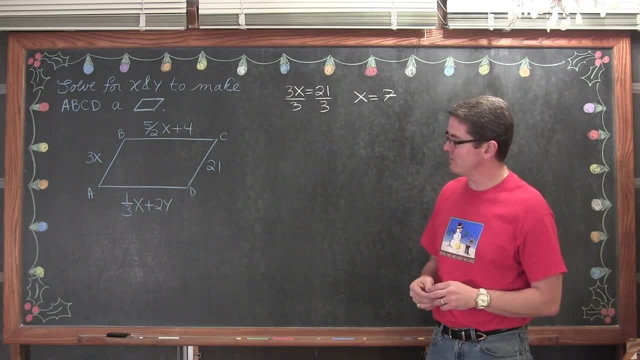 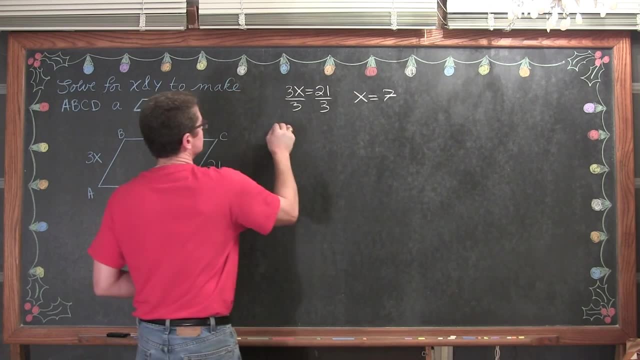 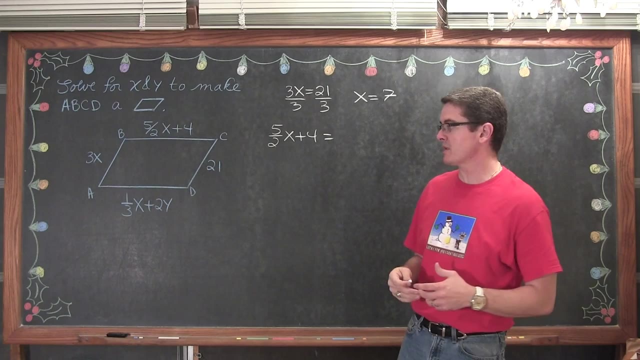 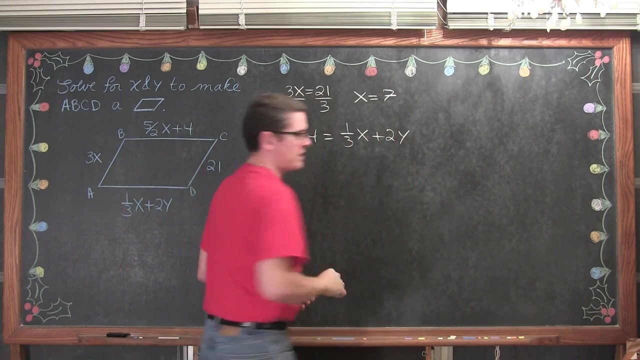 are congruent. Now I just need the other pair Subtitles by the Amaraorg community of size to be congruent. Our values here, our expressions, are 5 over 2x plus 4.. That side must be equal to the opposite side, which is labeled as 1 third x plus 2y. Ok Now. 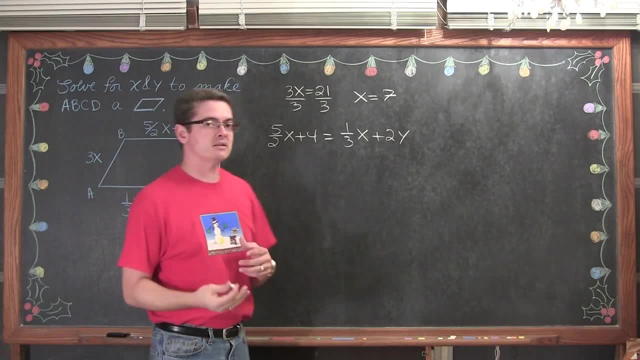 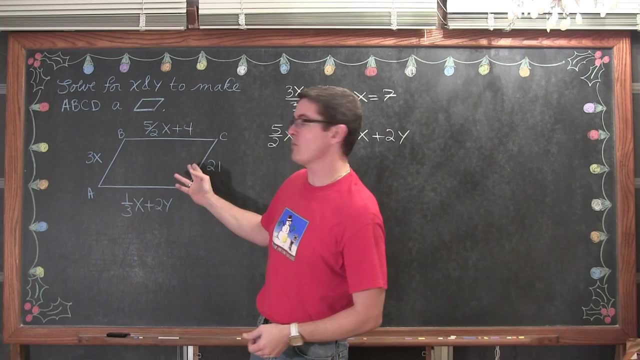 we have an equation here with two unknowns, which means that we can't solve for both variables at the same time. But thankfully I have got another diagonal within the same diagram, which means- or excuse me- not diagonal, but another pair of congruent sides. 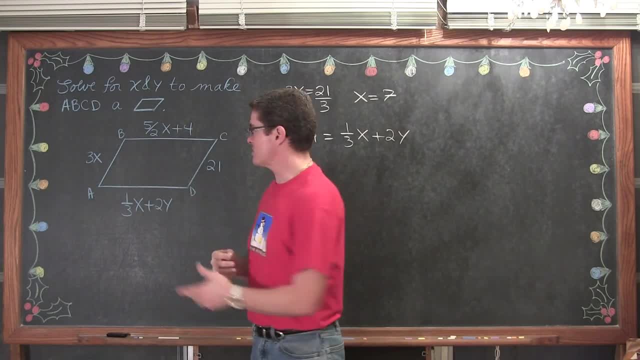 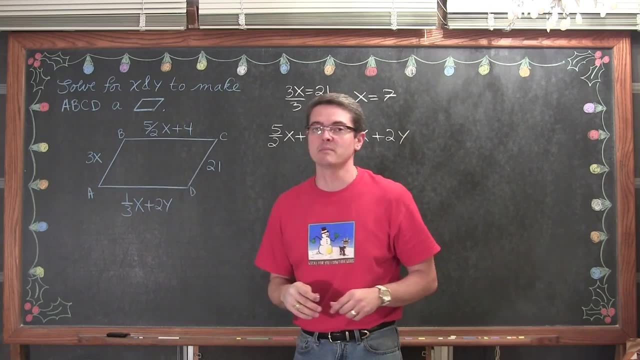 that I am going to force to be congruent in this diagram so that it is all related. So I have some information involving x from the fact that 3x must be equal to 21 for us to have any hope that this ends up being a parallelogram. I am going to use that information in a minute. 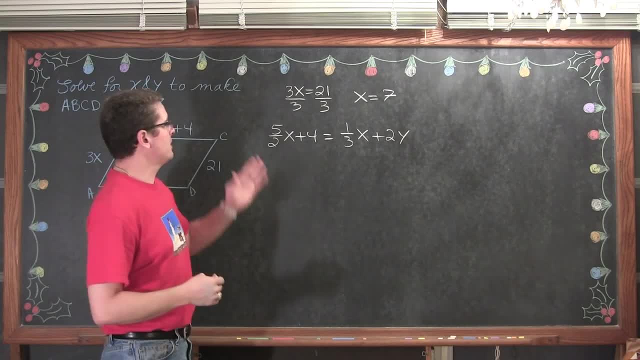 but first I want to clean this up a little bit and remind you again that if you have an equation with fractions, you can deal with it in a very simple way. You can deal with those all the way through. Find your common denominators when you are adding or subtracting. 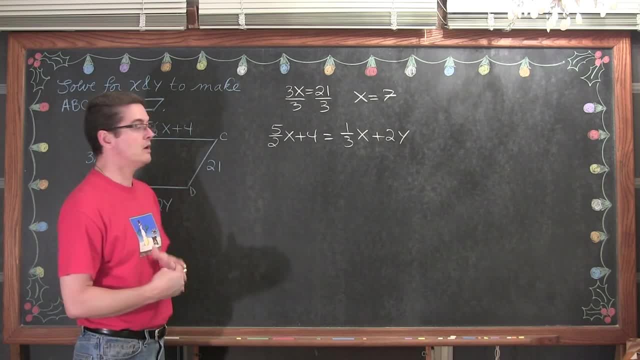 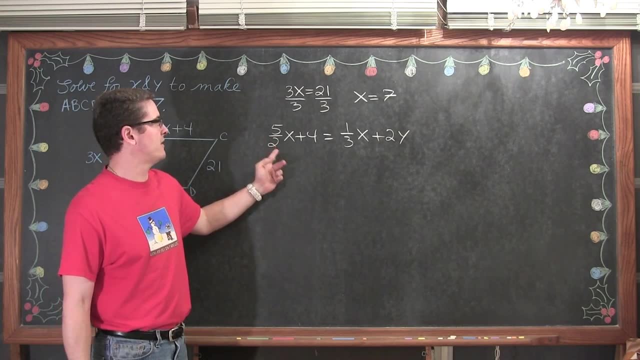 and deal with them however you need to when you multiply or divide, Or you can get rid of them right from the start. And I am not talking about doing 5 divided by 2, which is kind of ok because it is only 2.5. But 1 divided by 3 is a run on decimal, You know. 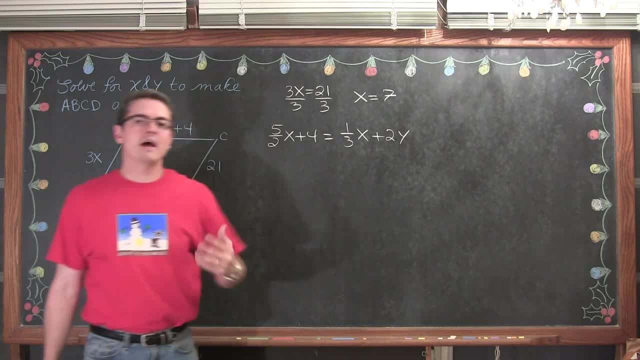 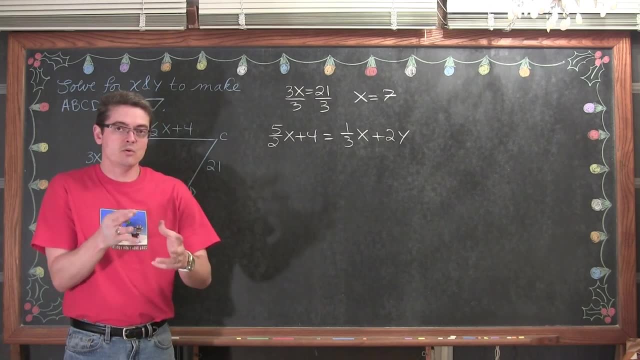 .3333333333.. So you are going to have to round off that value right from the start, which can throw off your answers, And that is not good. if you are taking a multiple choice test and you get a rounded off version and all the answers are not going to count in the 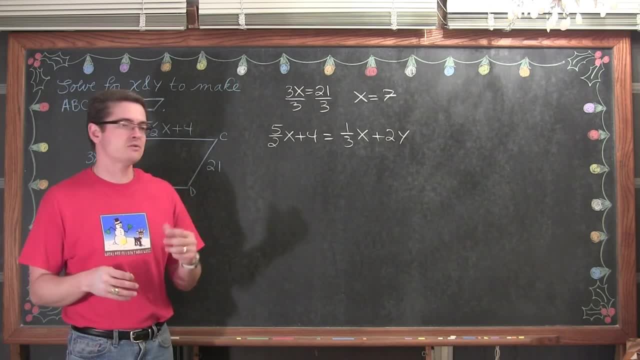 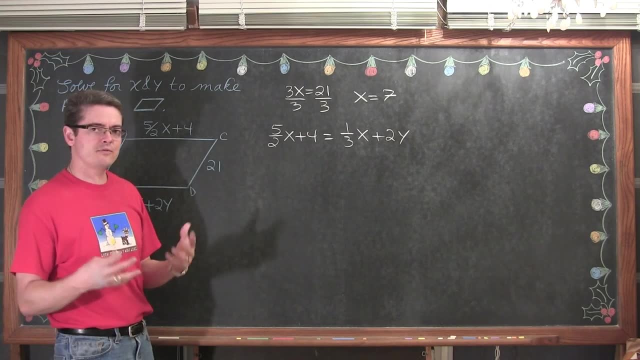 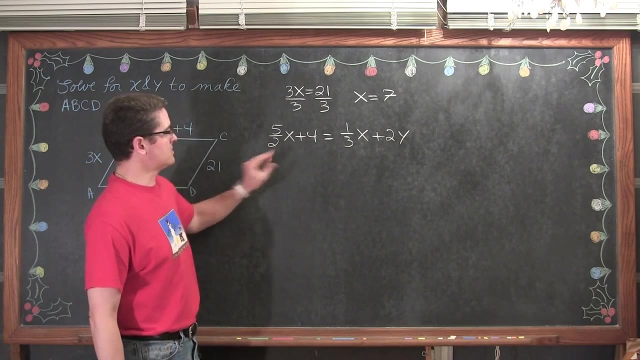 are an exact format and you don't get that exact match because you have made .3, repeating just .3 or .33.. So we want to get rid of those fractions, and even I like to work on my fractions, but they still lengthen the problem. So I want to look at our denominators of two and 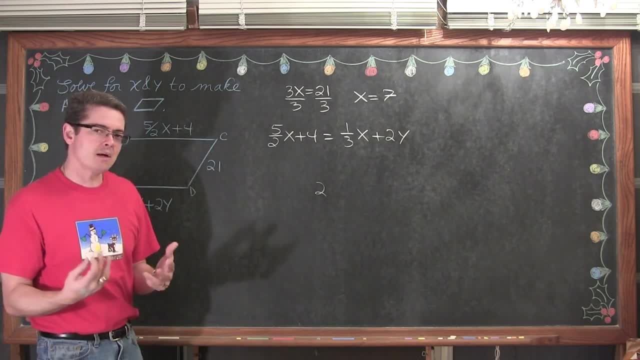 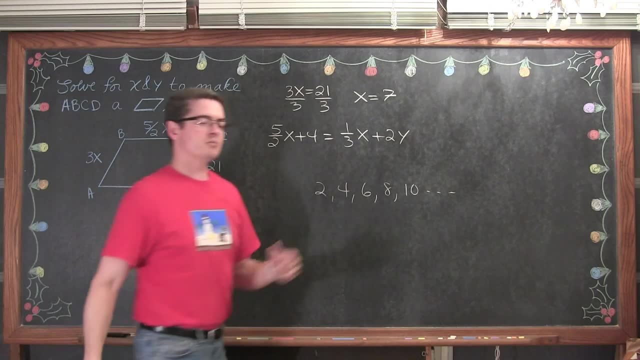 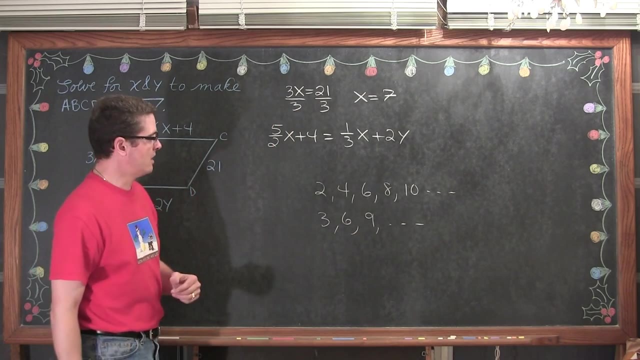 three and I want to find the lowest common multiple. We have two, four, six, eight, ten and so on. The multiples of three are 3,, 6,, 9, and so on, 12,, 15,, 18,, whatever, But 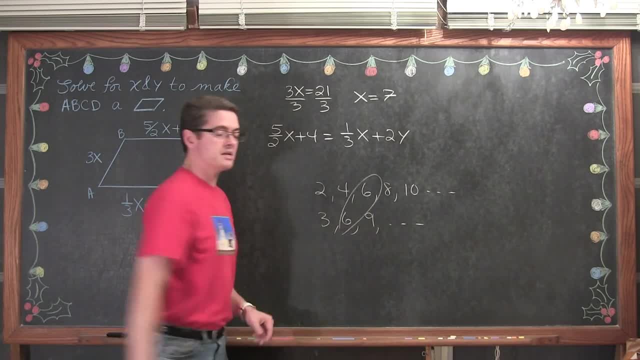 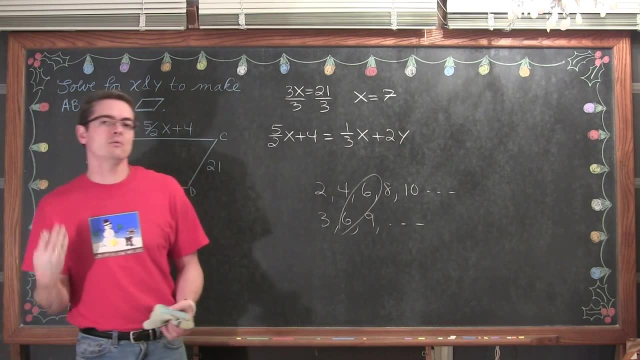 if I multiply by the lowest common multiple, which is six, then I can get the fractions out of my equation right from the start. It's going to add a step to my work but also make it a little bit easier by getting rid of our fractions. So we are going to multiply everything. 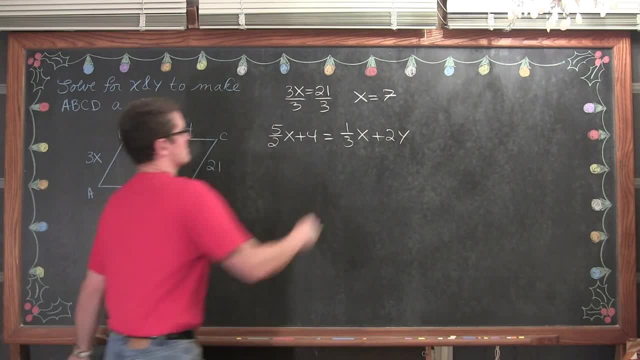 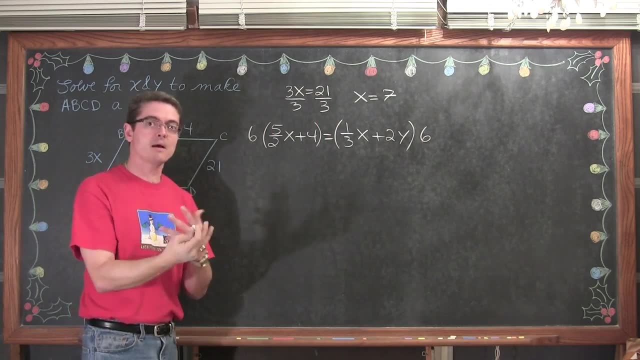 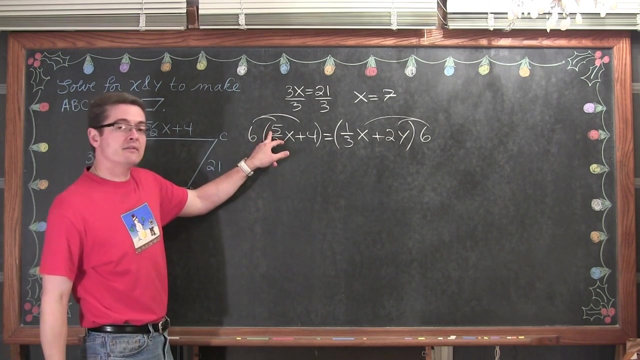 by six. So I am going to multiply the lowest common multiple six and then I'm going left and the right side of our equation by 6.. You can basically do anything you want, as long as it is the same math operation on both sides. We have 6 times 5 is 30, and 30. 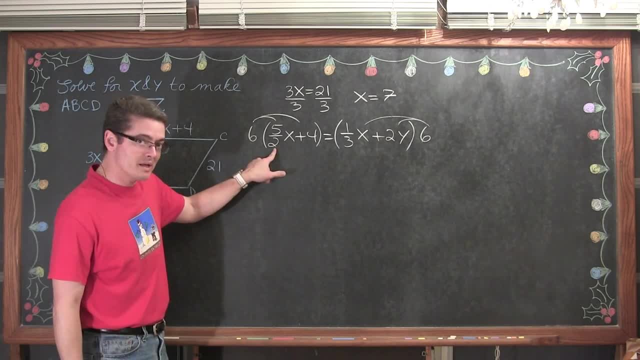 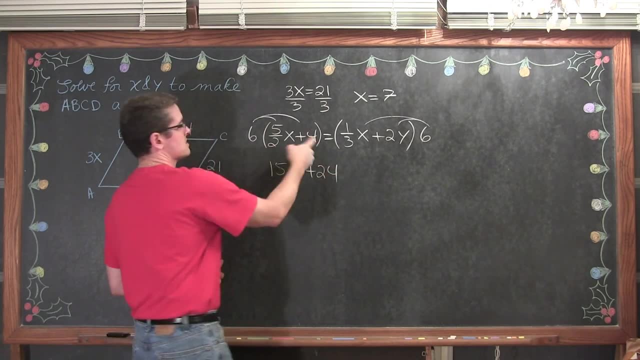 divided by 2 is going to be 15.. Or 6 divided by 2 is 3, and 3 times 5 is still 15.. So we have 15x plus 24, I am doing 6 times 4, and that is equal to 6 divided by 3, which is 2.. 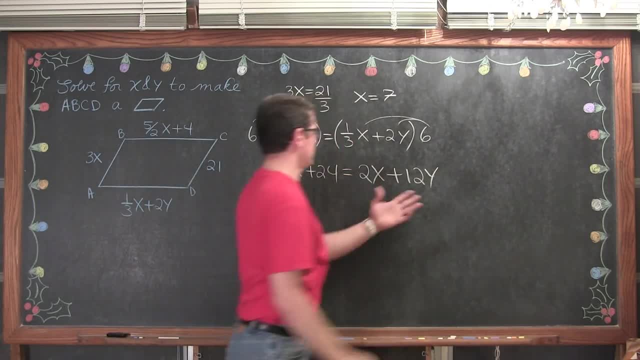 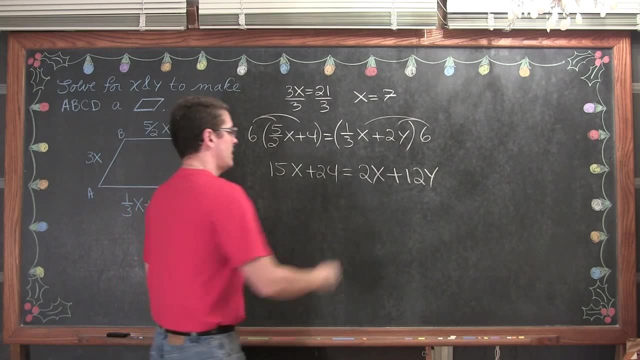 6 times 2, which is 12.. Now we are here. I am trying to solve for y, so I am going to get the x's together on the same side. I want to move this positive 2x over to the left. 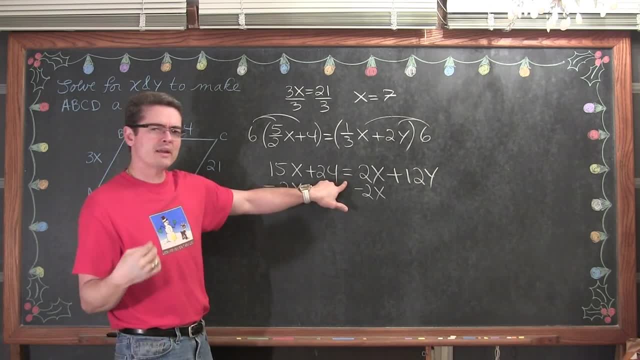 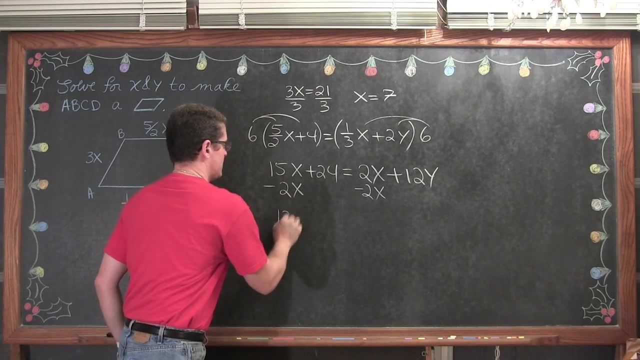 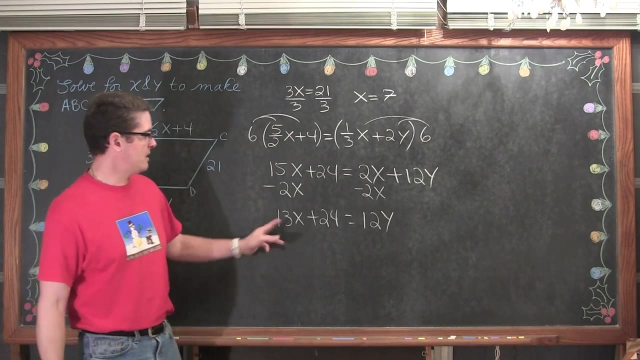 hand side of our equation. Whenever you cross that equation or that equal sign of the inequality you want to do that. We are going to do the opposite math operation. so we are going to subtract because it is already positive. We get 13x plus 24 is equal to 12y. Now to finish this up again, I have 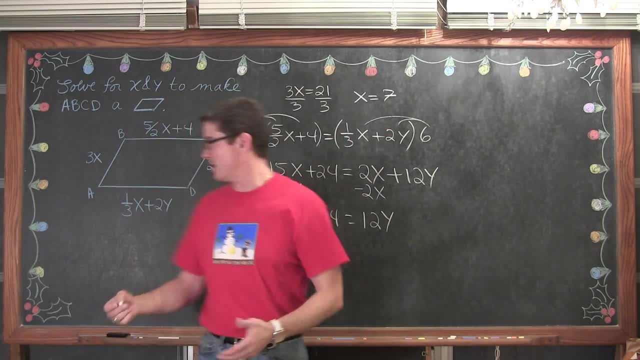 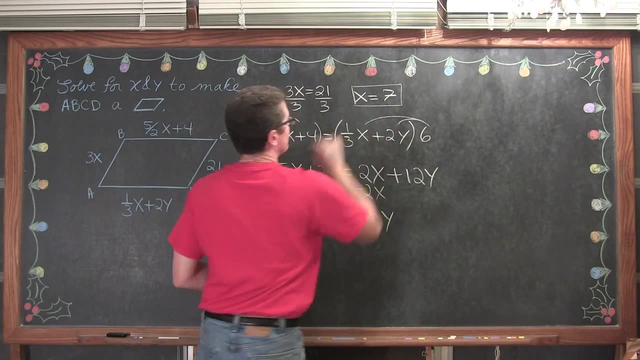 two variables, but I already know from the previous problem, or the previous set of opposite signs, that x is equal to 7.. So I am going to take this value and basically do the substitution method for solving a linear system of equations. This is a linear equation I am going to do. 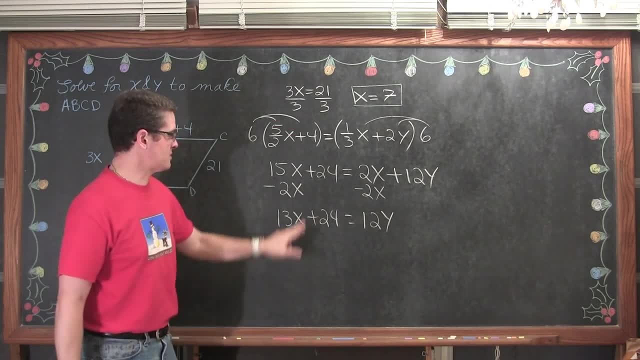 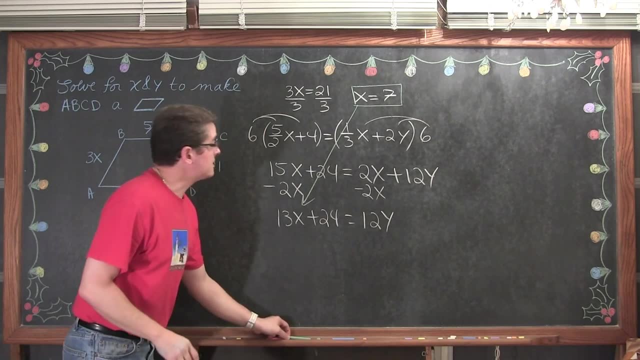 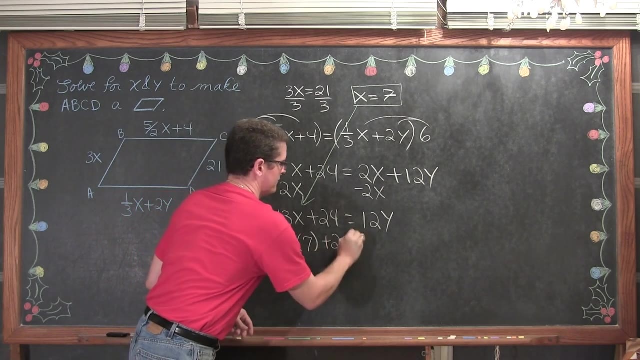 a linear equation. It has an exponent of 1.. This is a linear equation because we only have exponents of 1 here and our unknown values. So we are going to plug that value of 7 in for x and we get 13 times 7 plus 24 is equal to 12y. Let's see: here We have 10 times 7. 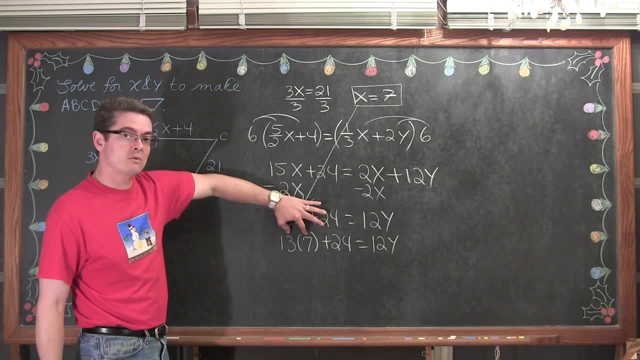 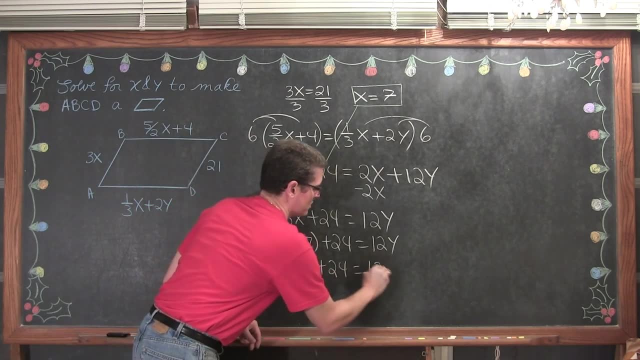 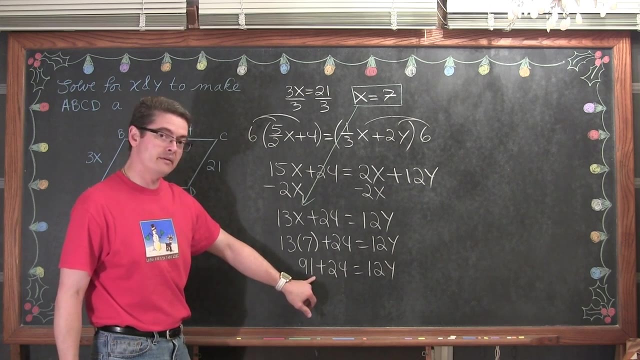 which is 20, or, excuse me, 70. We have 7 times 3, which is 21.. So we have 70, and 21 makes 91.. Plus 24 equals 12y. We have 91 and 24.. Well, 90 and 20 is 110, now we are at 111,. and now 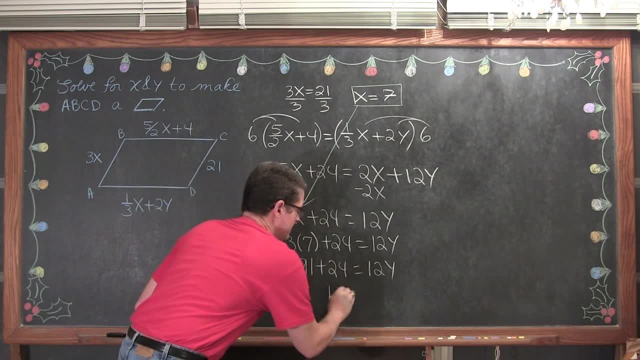 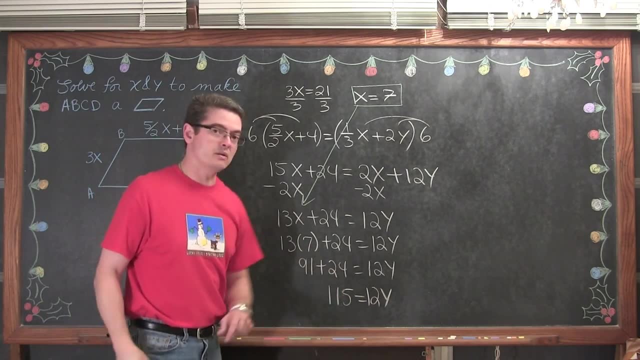 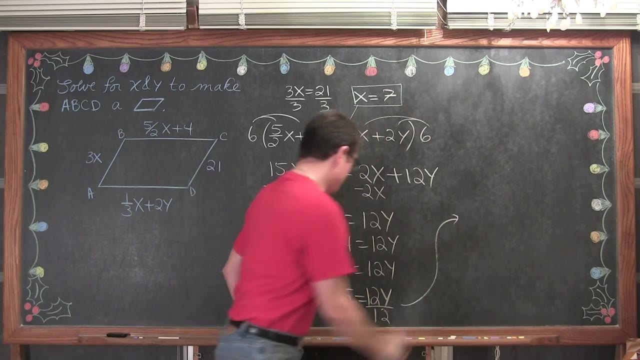 we are at 115.. So we have: 115 is equal to 12y. I want to get that 12 away from the y. I am going to do that by undoing the multiplication. by doing the inverse math operation of division, We get a y value. 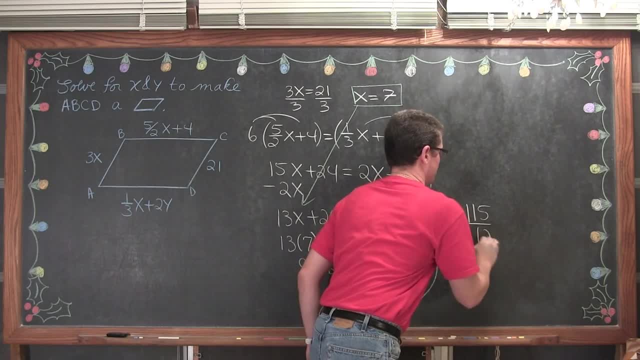 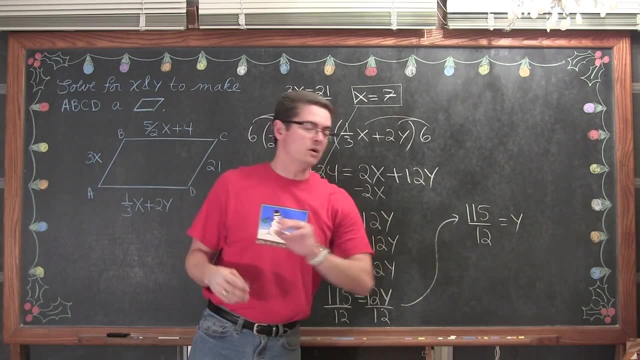 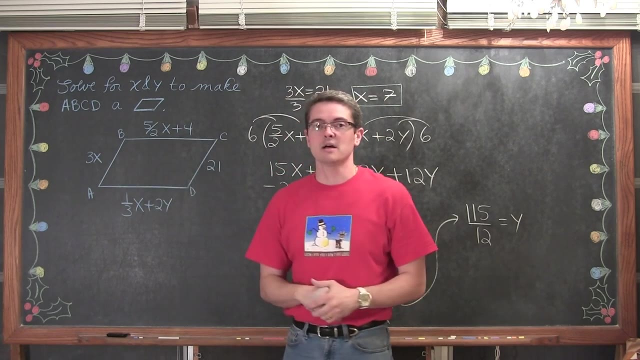 We have a y value of 115 over 12.. Now that fraction does not reduce, so that is our final answer. We have an x value of 7 and a y value of 115 over 12, which will ensure that this is a parallelogram. That means the opposite sides, both pairs of the opposite sides again. 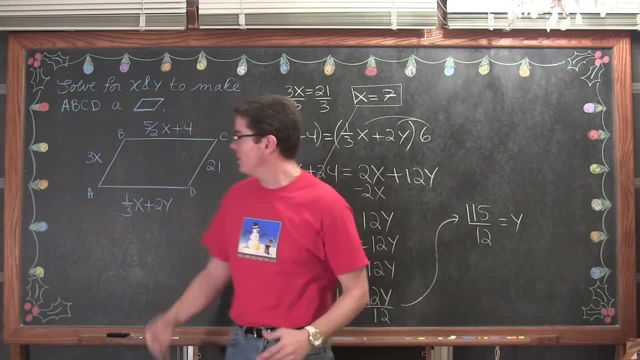 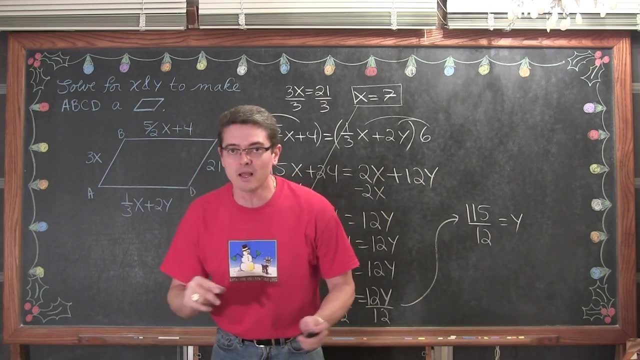 have to be equal. If you want to check this, you are going to plug the values of x and y into these expressions and make sure that the opposite sides are equal. But I am instead going to do that by undoing the multiplication, by doing the inverse math operation of division. 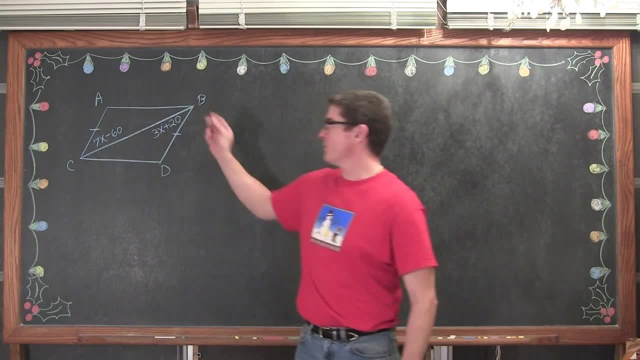 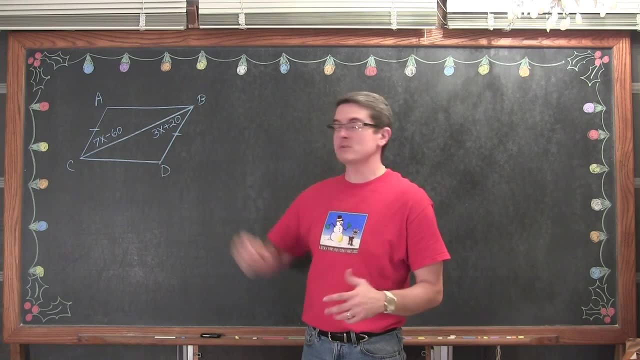 Here we have another quadrilateral, Only this one has a diagonal going through it of bc. We want to again find values of the unknowns. In this case we just have x, So we are going to solve for x in such a way that we are going to make sure that this quadrilateral is indeed. 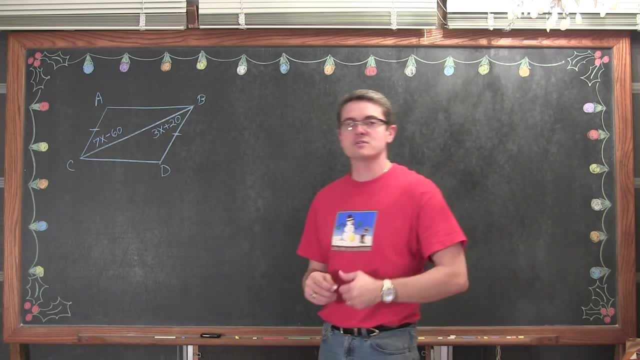 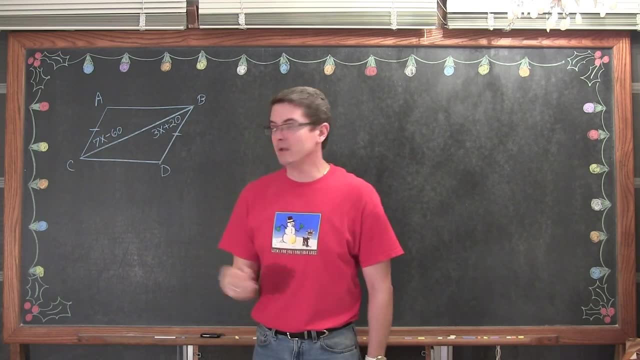 a parallelogram. Now again, one of those converse theorems we just looked at said that if you have one pair of opposite sides- Opposite sides which are congruent- and we have those marks in there, If they are parallel, then we have enough information to state that the entire quadrilateral is a parallelogram. 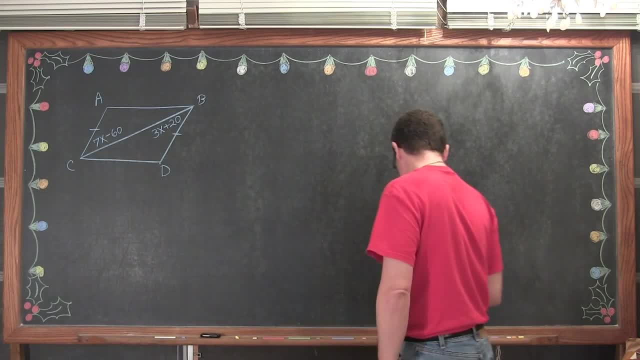 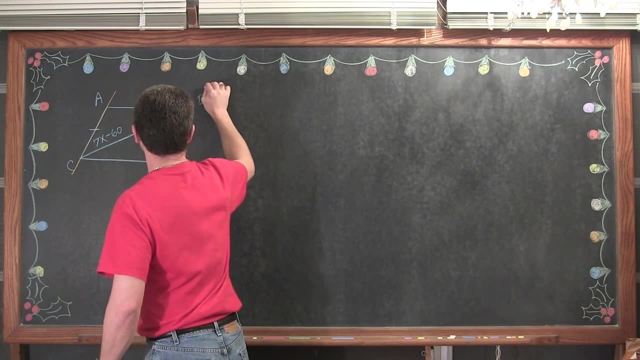 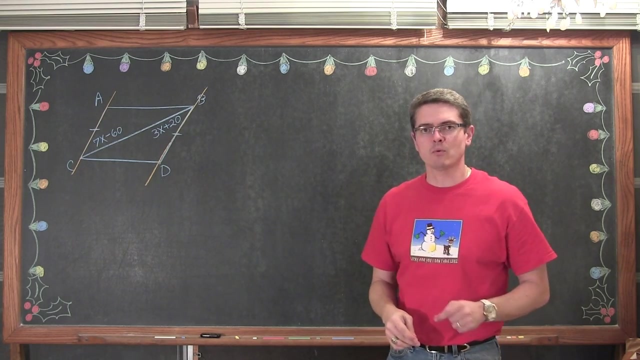 So we have congruency again. So all we have to do is show, let's see here- that this side is parallel to this side, That ac is parallel to bd. Now I am kind of highlighting just what we are focusing on here. 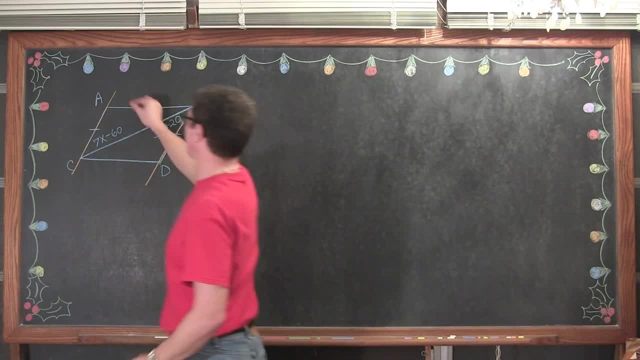 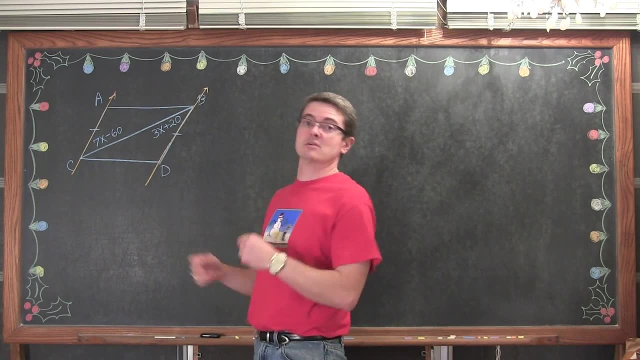 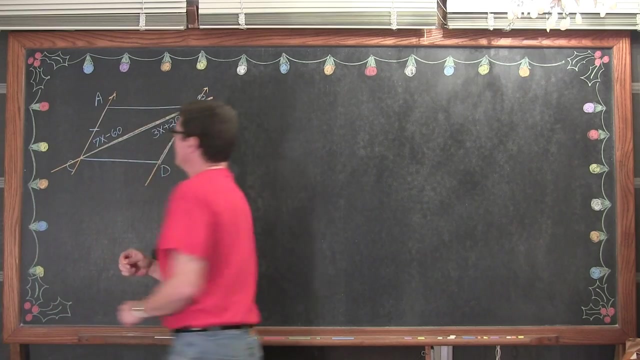 Remember back when we started studying parallel lines, that when two lines that were parallel and that is what we are trying to force to happen. So maybe I should just say it in the converse: If two lines are cut by a transversal, so then two lines cut by a transversal. if 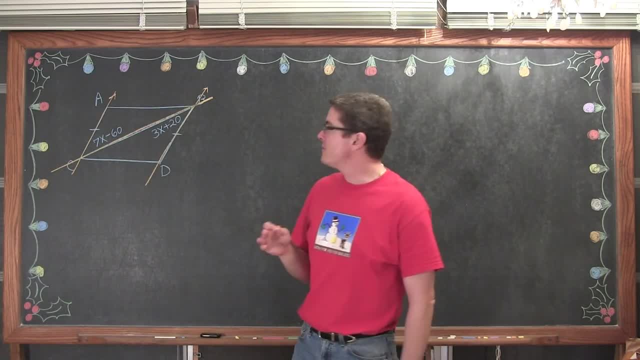 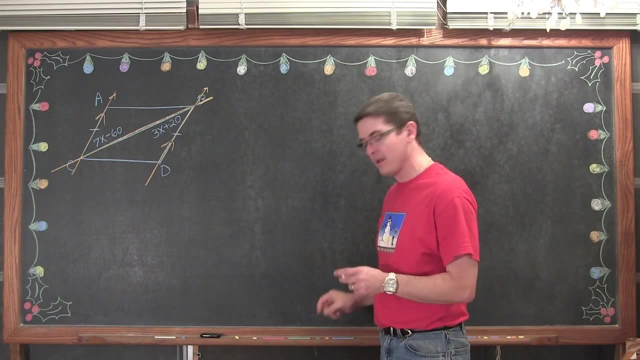 the alternate interior angles are equal, then those lines, indeed, are going to be parallel. So what we are going to do is make sure that we have a parallelogram, So we are going to make sure that those alternate interior angles are equal by setting them equal. So 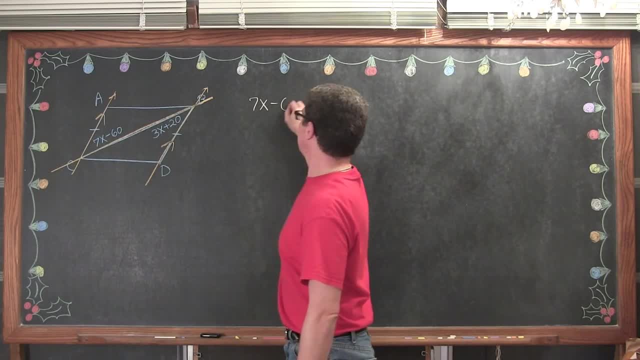 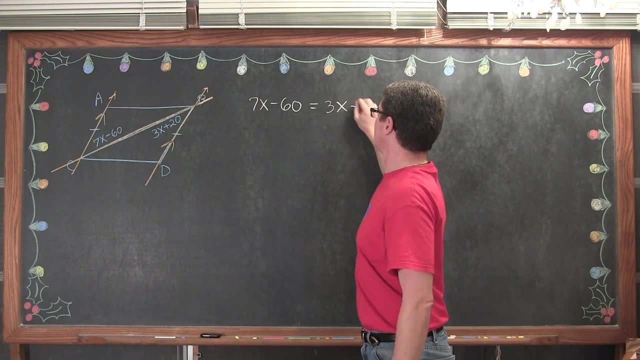 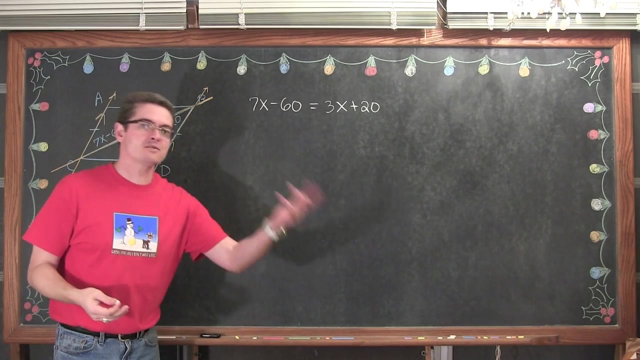 we have 7x-60 and that entire expression is representing the number of degrees of this angle. We are going to make that equal to 3x plus 20.. So really, again, we are doing the same thing we did in the past video. only in the past video, the previous one, we were. 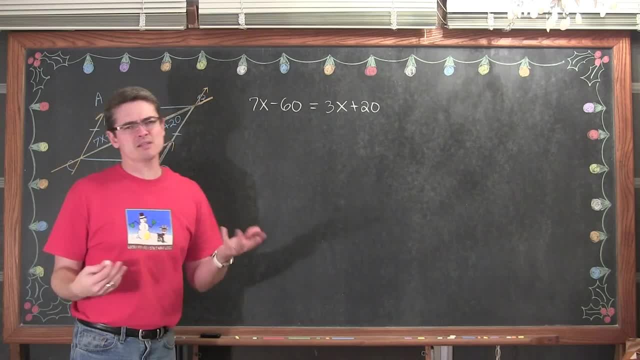 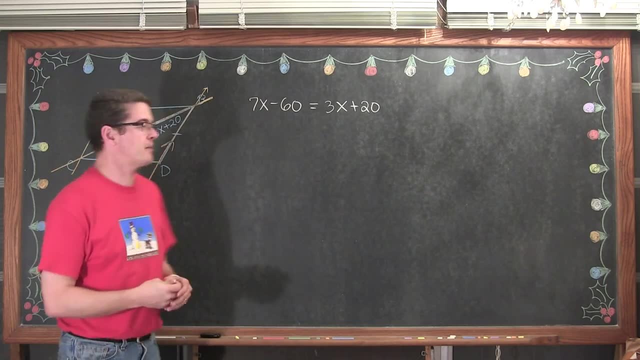 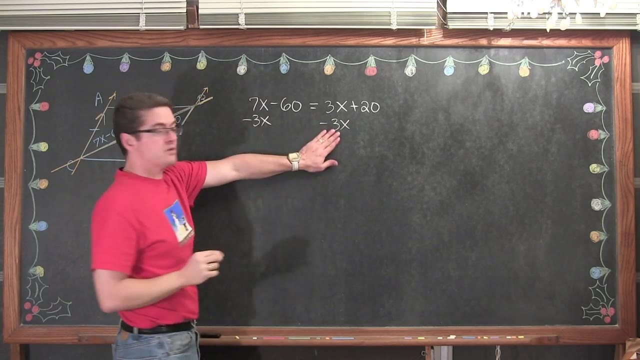 told that it was a parallelogram, so that we knew that these were equal. This time we are setting them equal to make sure That we have the proper properties to state that it is a parallelogram. So we are going to subtract both sides by 3x, trying to undo that positive 3x and move it over to the left. 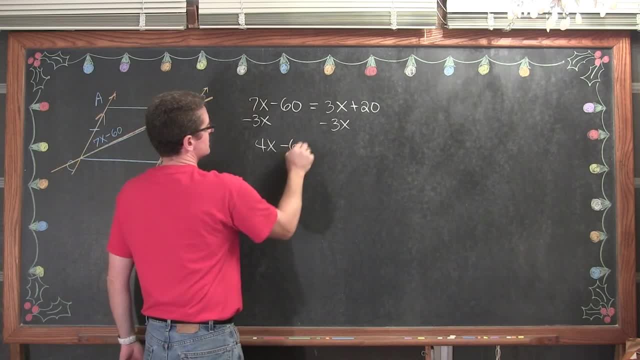 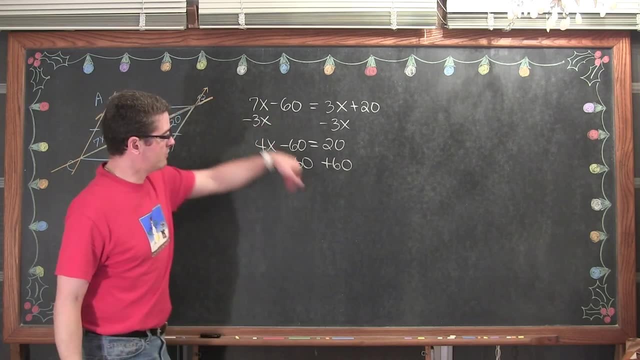 We have 7-3, which is equal to 4x. minus 60 equals 20.. We are going to add 60 to both sides of the equation, moving it away from the x, which is now on our left. The opposite of subtraction is addition. We are going to add 60 to both sides of the equation, moving 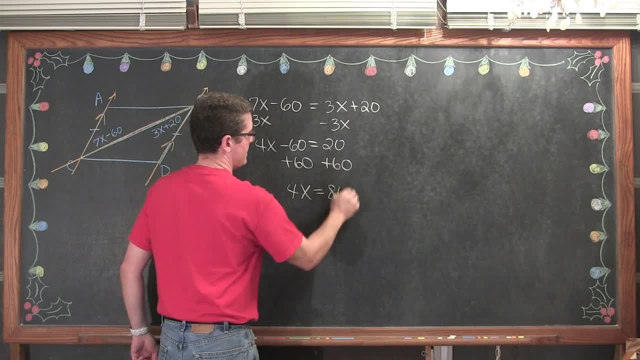 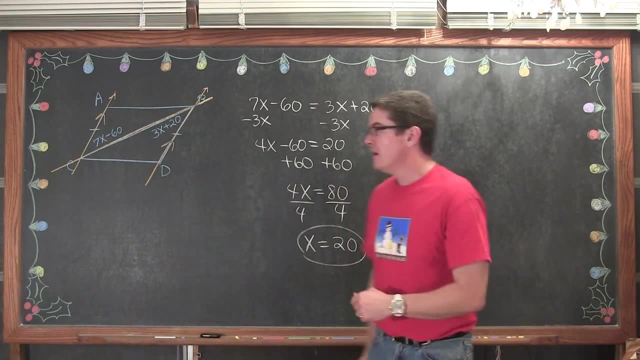 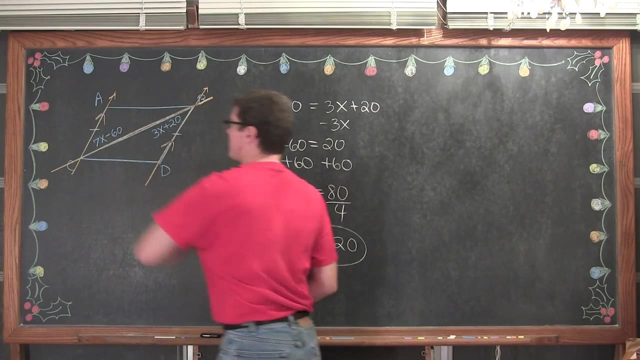 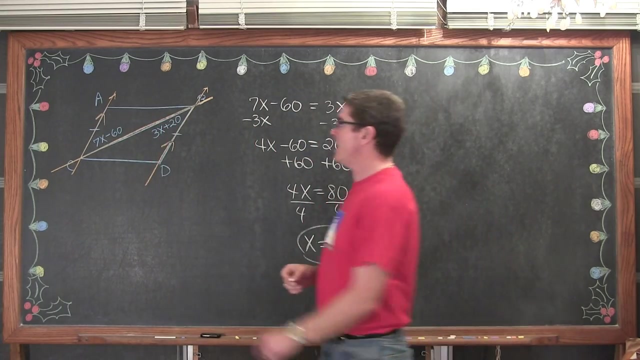 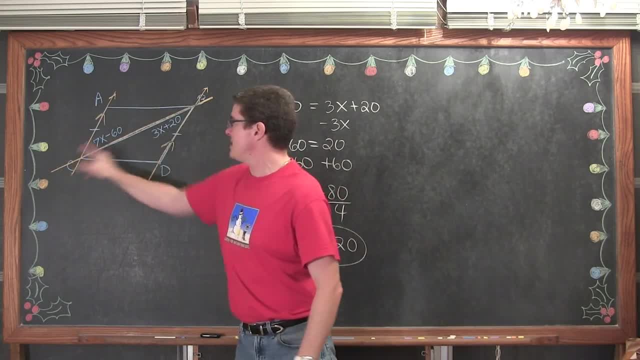 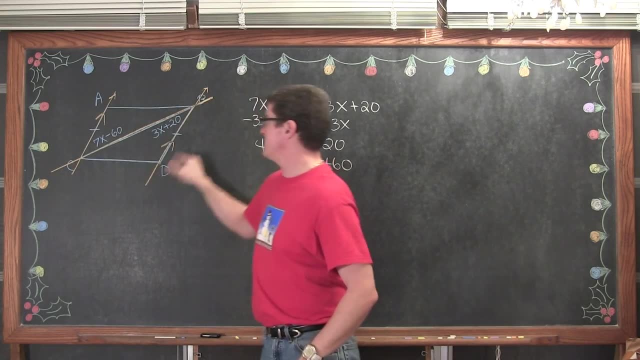 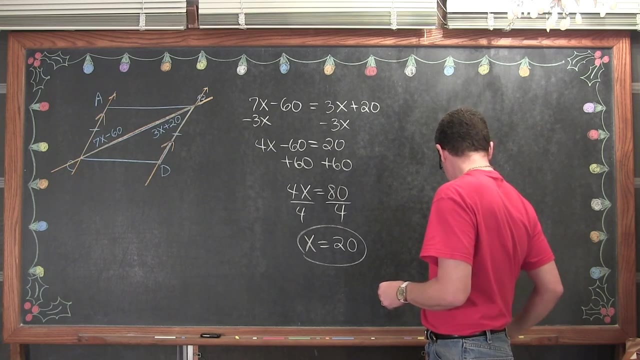 to be- or excuse me, not ABCD, because I just ran through the middle of my parallelogram, but that ABDC or ACDB is a parallelogram. If I want to actually know the size of those angles, then let me get some purple chalk. here We are going to take this value of 20,. 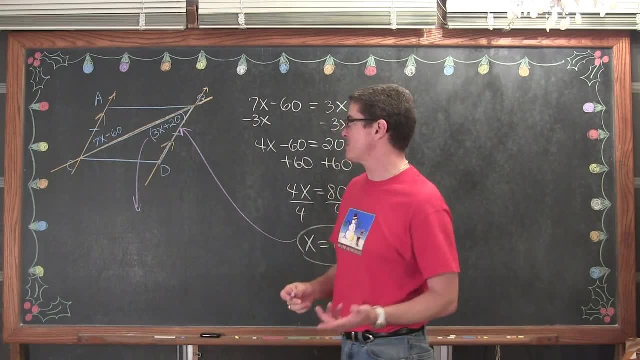 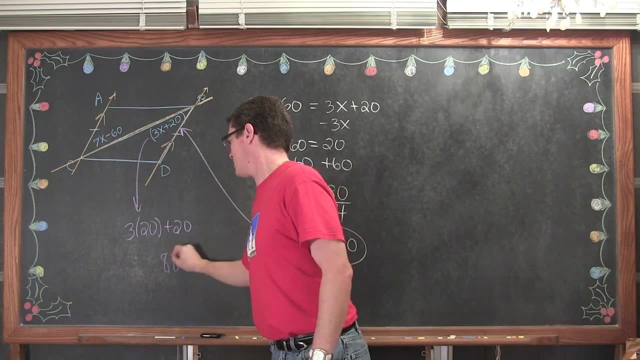 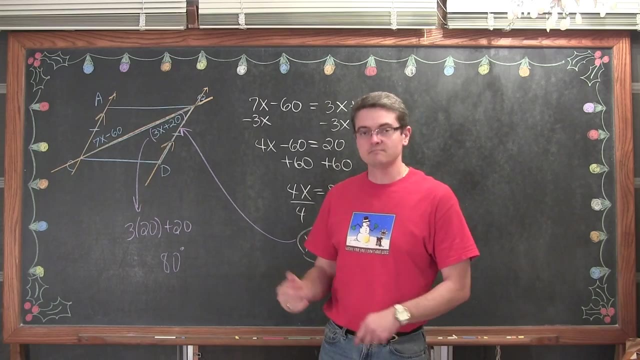 plug it into the expression that represents the amount of degrees that angle represents, and we have 3 times 20 plus 20, well, that is, 60 plus 20 is equal to 80 degrees. Alright, our last example is going to be a two column proof and we are going to, well, just get. 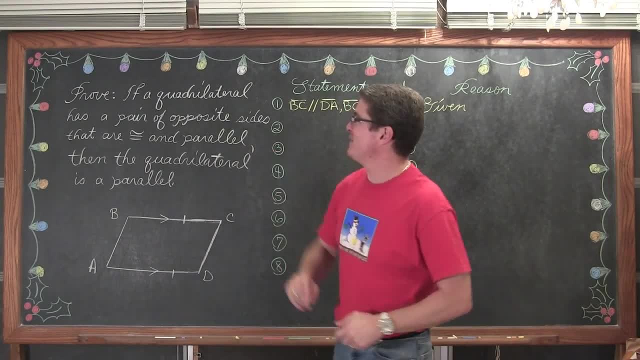 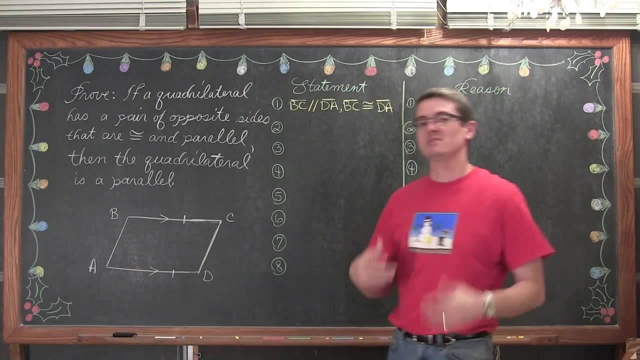 to it right now. Woo, Love me some proofs. Alright, if a quadrilateral has a pair of opposite sides that are congruent and parallel, then the quadrilateral is itself a parallelogram. So we have a quadrilateral ABCD and we have a quadrilateral ABCD And we have a quadrilateral. 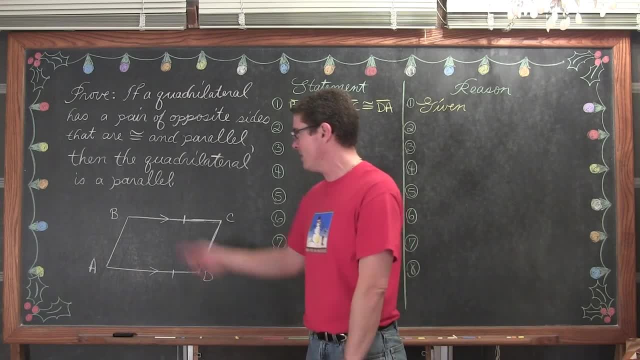 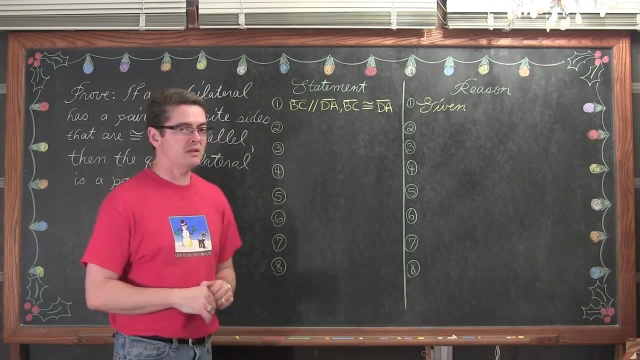 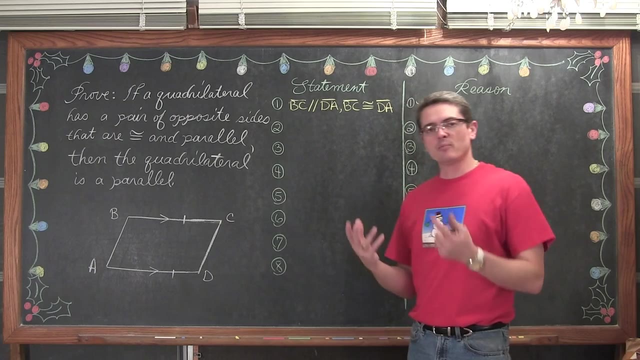 ABCD and we have the opposite sides which are parallel and congruent. So BC is congruent to AD and those same two sides are parallel and we have it up here as given information. Now, if we think back so far we have studied in geometry, we have had done a lot of proofs. 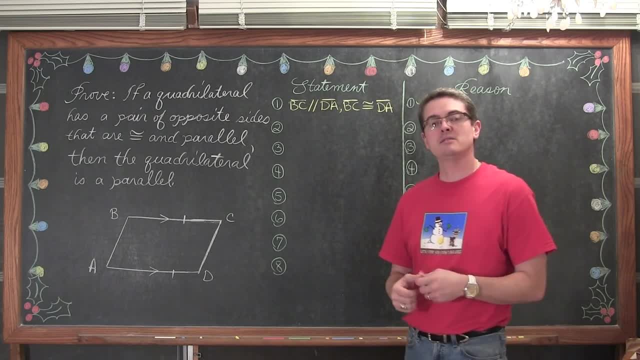 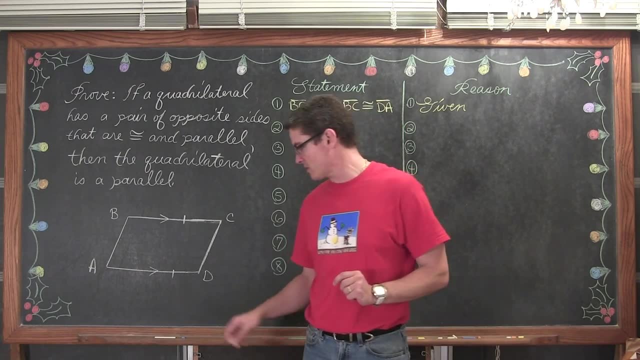 on proving things dealing with parallel lines, and we had a lot of proofs where we dealt with proving that two triangles were congruent Subtitles by the Amaraorg community. Now what we want to do is, ultimately- I am going to make this little proof a little bit- 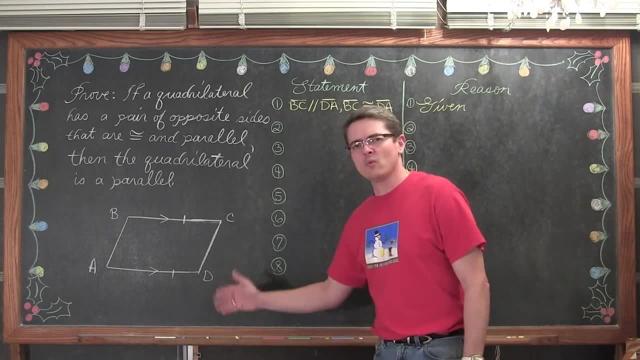 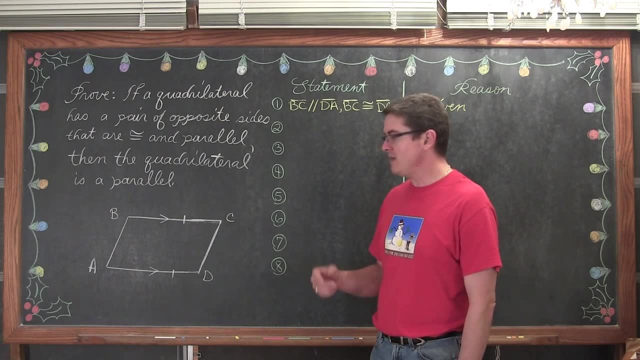 longer than it needs to be. I have not done one in a while, So we are going to go all the way down to the definition of a parallelogram, which is: the opposite sides are parallel, both pairs. So we need to add something to this diagram and it is going to be basically: 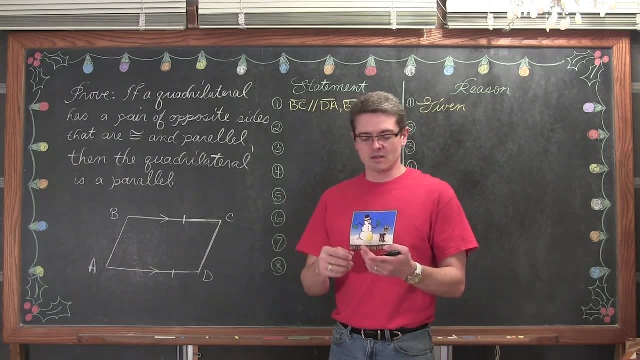 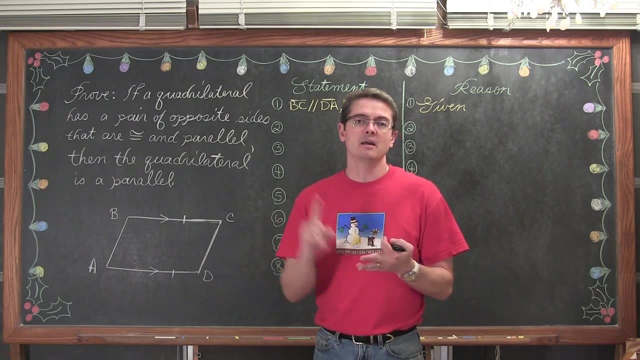 what we know a lot about, which is triangles. We have got four ways of proving- well, really five. if you want to conclude, right triangles We have side-side-side, side-angle-side, angle-side-angle- I don't think I said that yet- And if the two triangles are right triangles we have 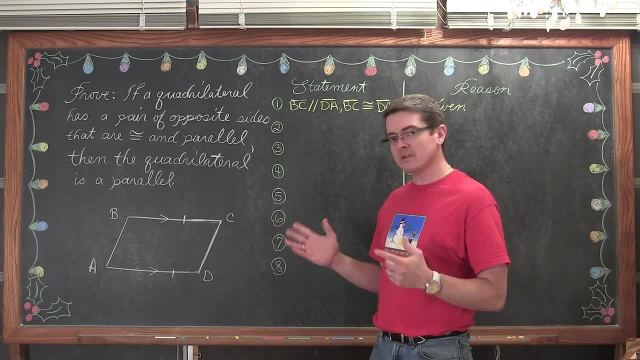 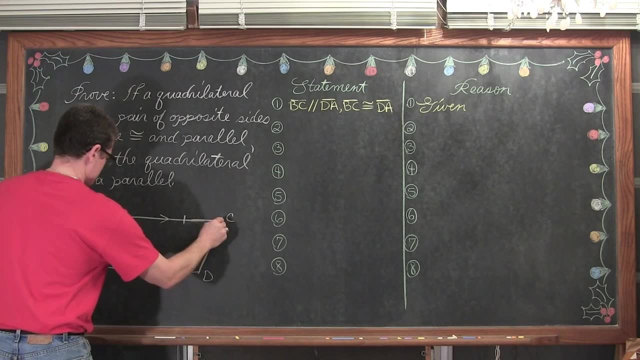 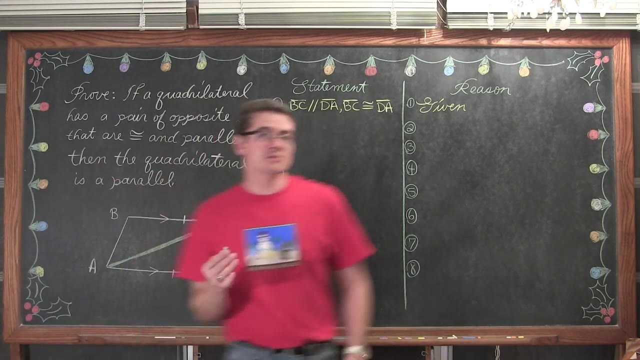 hypotenuse leg. Now we are going to basically, let's see, here I want to add a diagonal, and so we are going to do it here from C to A- A little crooked there, Ok. So we have diagonal CA. Now what we want to do is I want to ultimately prove that these two triangles are congruent. 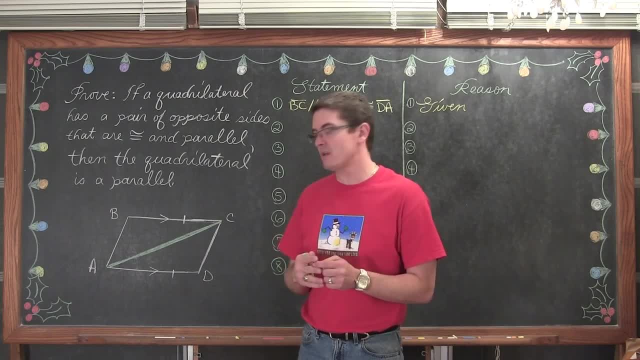 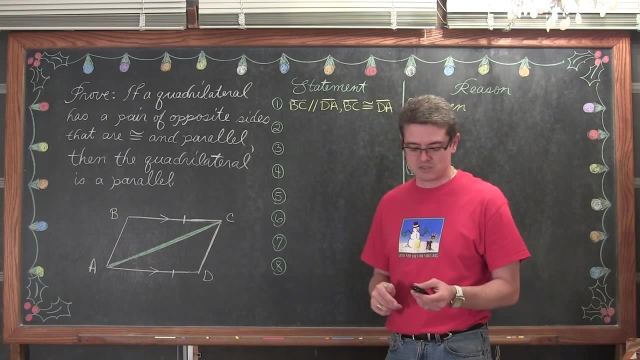 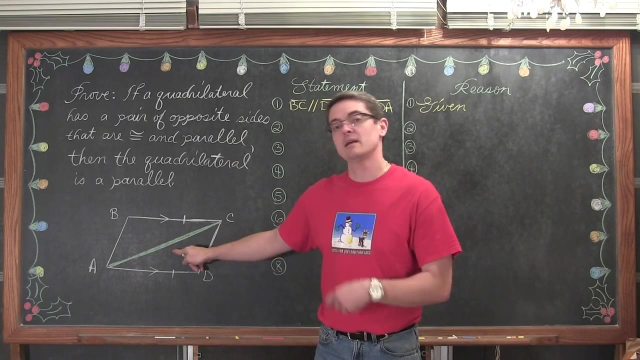 Subtitles by the Amaraorg community. That is going to help me fill in some information that is going to allow us to prove that AB is parallel to CD. But if I am going to prove these triangles are congruent, let's start with what is very obvious, which is I have two triangles now sharing a common side, a. 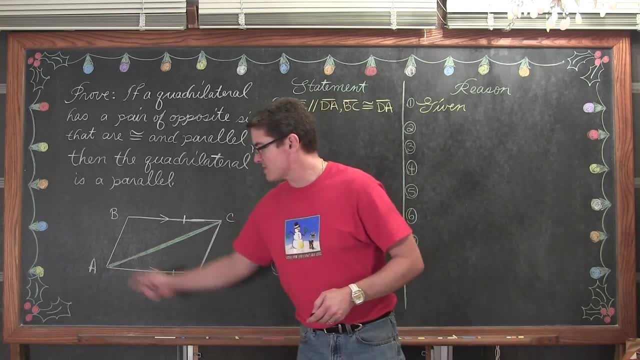 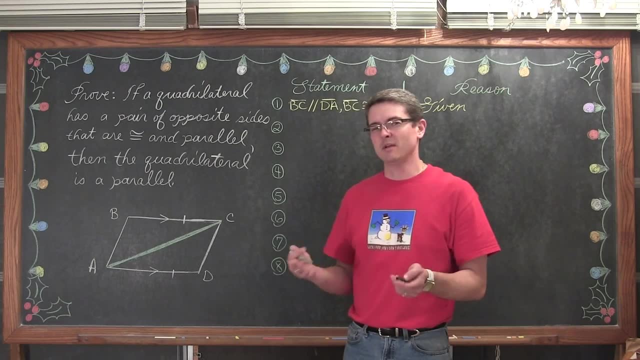 common diagonal of AB. So we are going to say that AC is congruent to AC. Again, we are saying that twice because it is now part of two separate triangles. It makes a bit more sense to say that something is equal to itself. So we are going to say that AB is congruent. 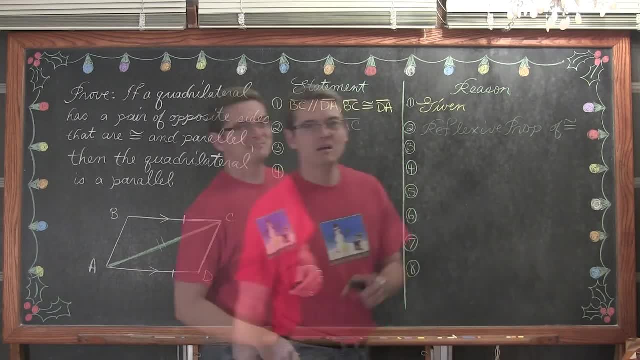 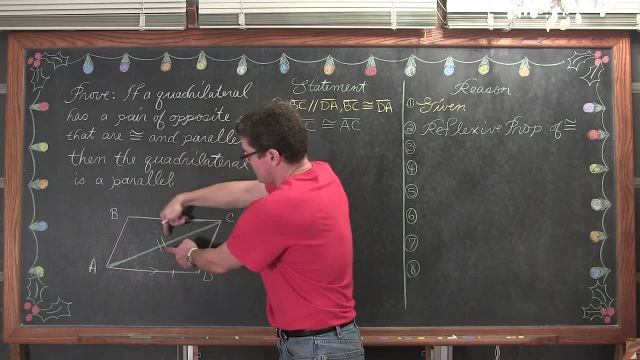 to AC. And again, we are saying that twice because it is now part of two separate triangles And we can also make that two side equal to itself. We are going to make that line 2.. Ok, So now we have a couple of triangles that have a pair of congruent sides and another. 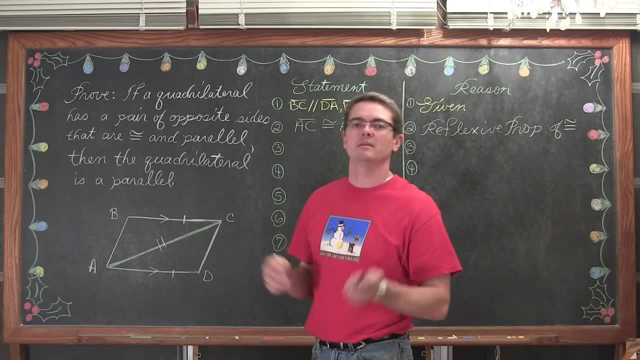 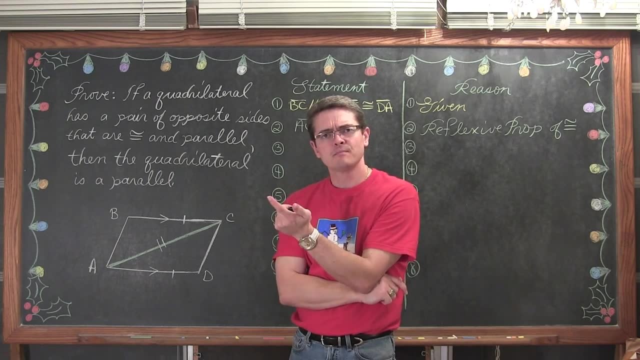 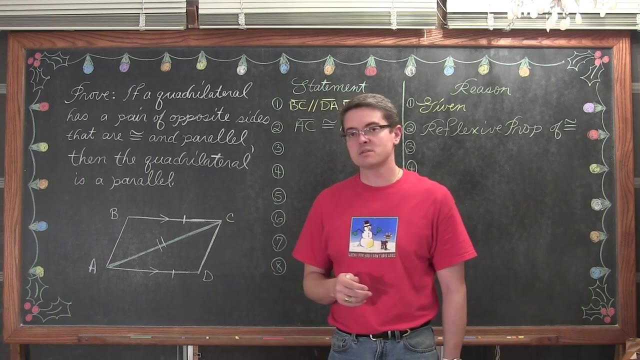 pair of congruent sides. But that is not enough. There is no side-side postulate for proving two triangles are congruent. So, um, any ideas? Is there any information on here that can allow us to fill in? let's say that the opposite sides here of AB are congruent to CD. No. 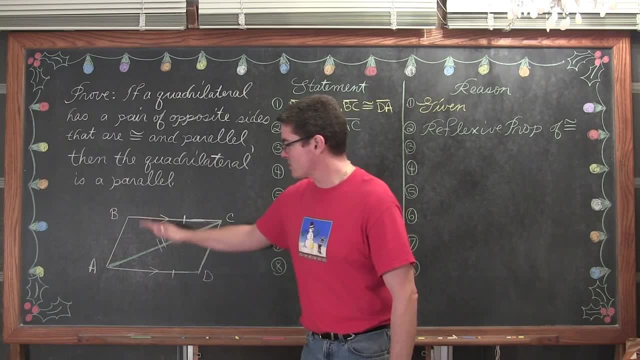 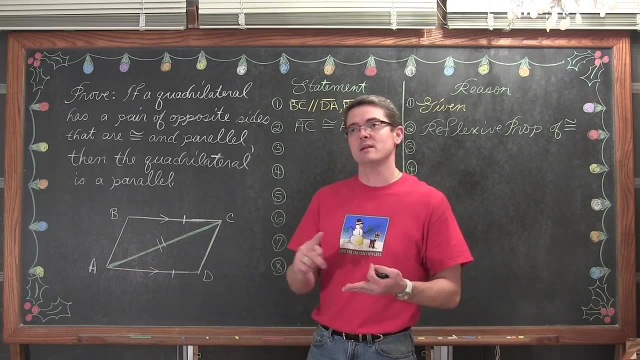 Um, But we do have two lines which are parallel. And again remember parallel lines. We had same side interior angles, which were supplementary. we had corresponding angles which were congruent. we had same side exterior angles which were congruent. and when we had 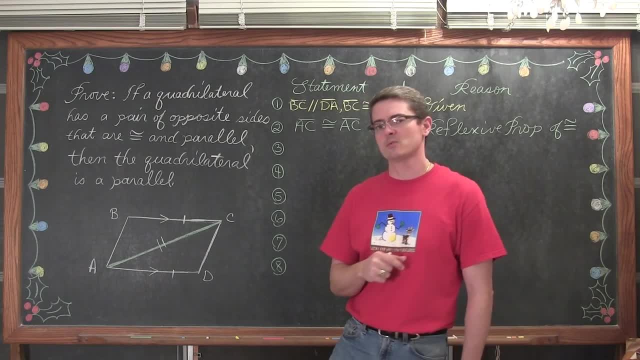 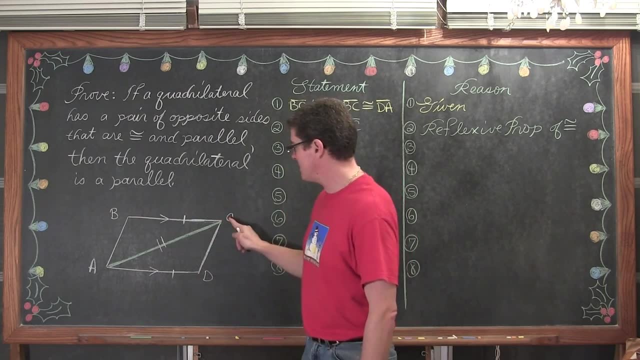 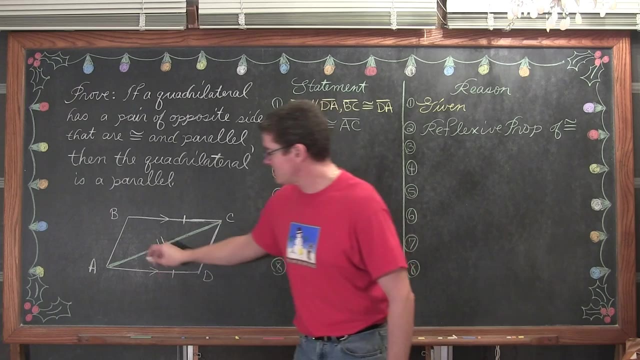 the Z shape we had alternate interior angles which were congruent. So parallel line, parallel line being cut by a transversal. that means that angle BCA can be said to be congruent to angle CAD. these alternate interior angles are going: 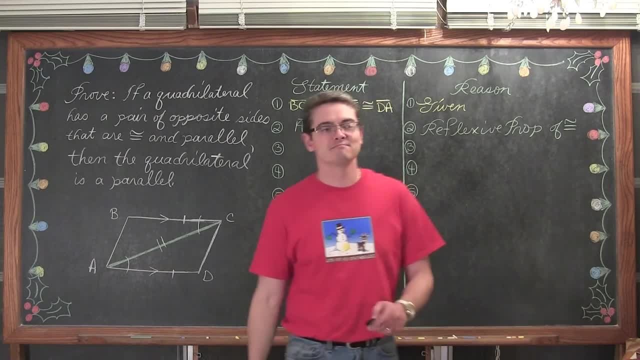 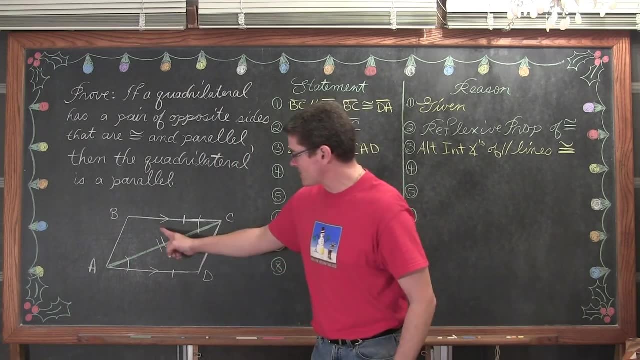 to be congruent because those two lines are parallel. There we go, BAM. Now I have already got that extra information into our diagram. Let's focus on these two triangles, remembering our four ways of proving non-right triangles are congruent. 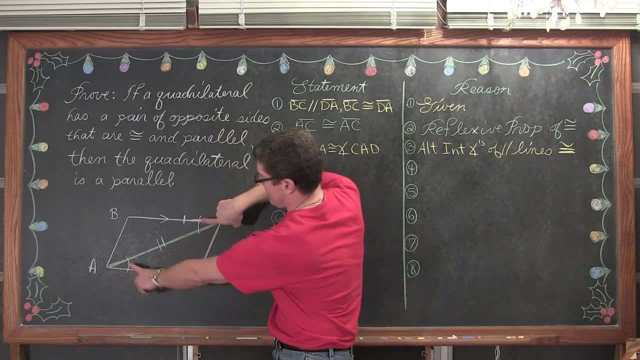 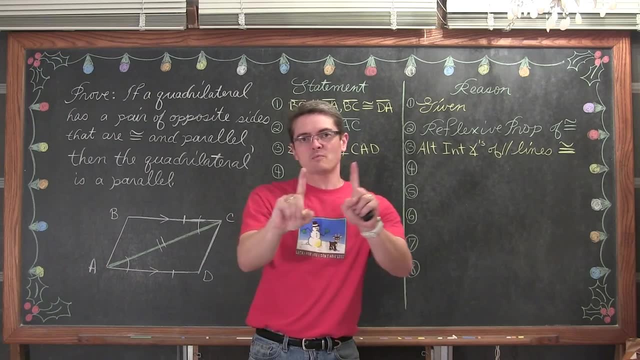 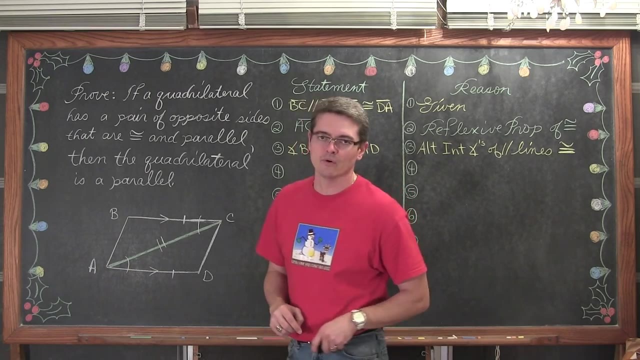 And we have side angle side. So let's name those two triangles and make sure that you have the congruent corresponding parts, in the same order, of both of your names And again, that is going to be side angle side for those two triangles being congruent. 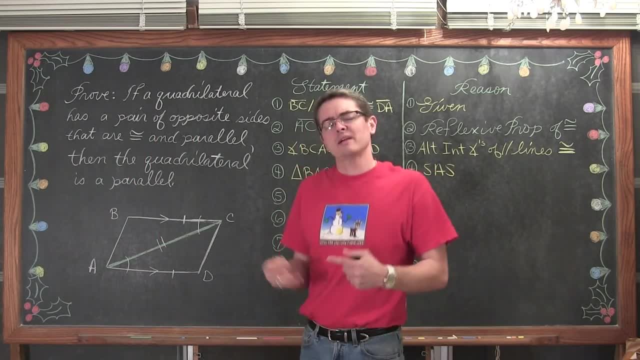 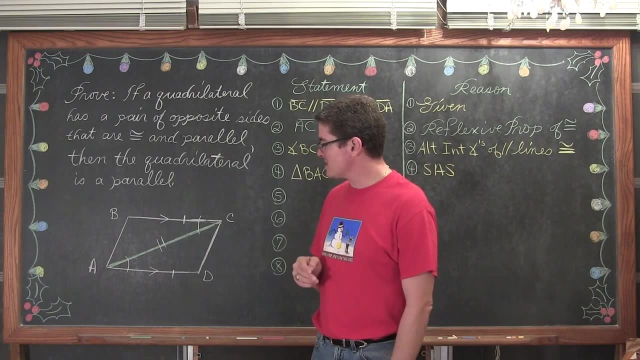 Congruent triangles. what do we like to talk about with congruent triangles? We like to talk about all their parts which are congruent as well. So if these two triangles are going to be congruent, we can say that. let's see here. 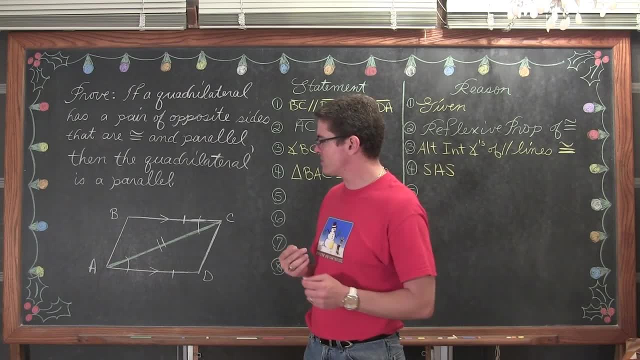 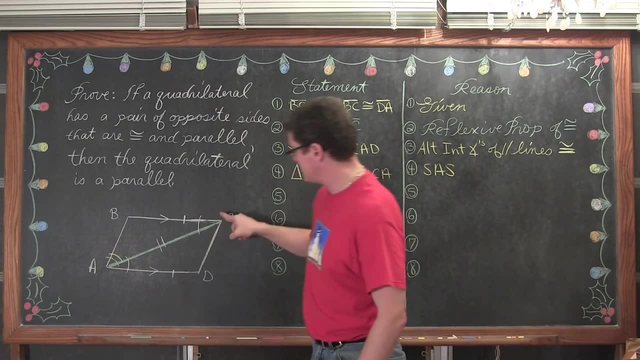 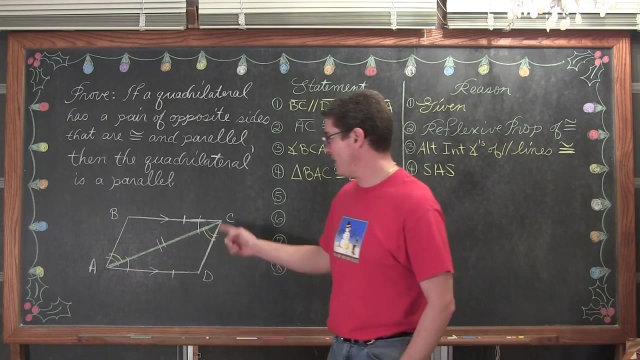 this angle and this angle. Why would we want to show that angle BAC is congruent to angle ACD. Well, I am not sure why I would want to, maybe yet hopefully you do, but they certainly are congruent because of- let's see here- congruent triangles and congruent parts which 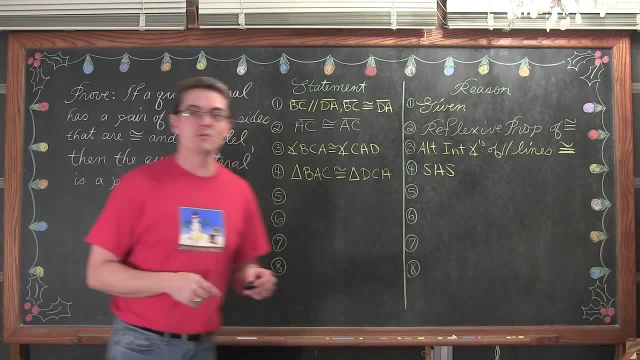 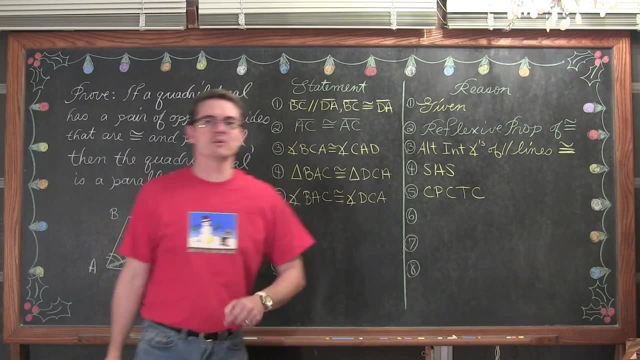 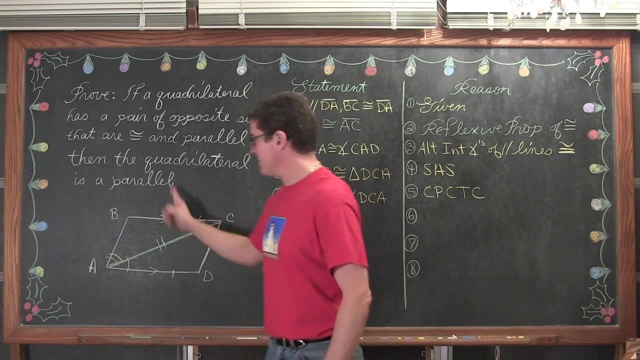 are congruent. That sounds like I have to use a bunch of letters to state my reason. Yes, that collection of letters is congruent. Yes, Corresponding parts of congruent triangles are congruent. So now that I have those angles being congruent again, I have two lines. 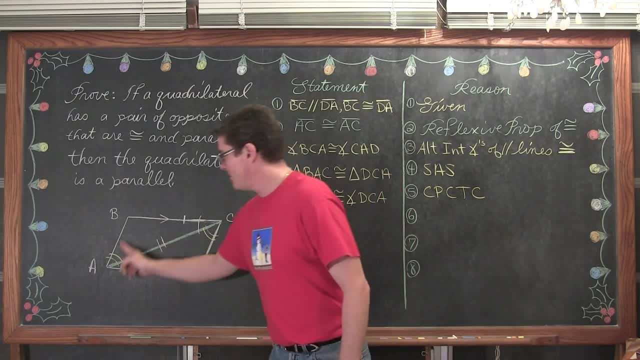 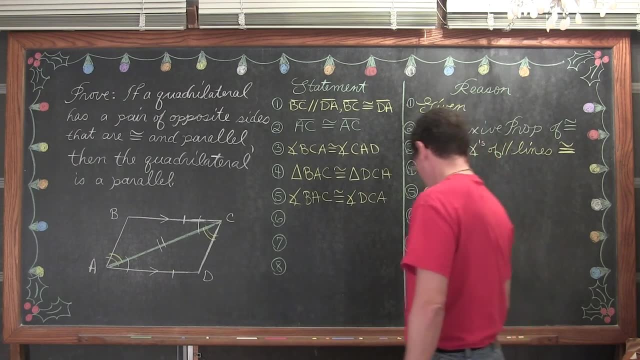 Now, this time, I don't know, my lines are parallel, but I do have two lines being cut by a transversal. and let's see, I know that my red chalk doesn't show up much on the camera, so we will do purple. 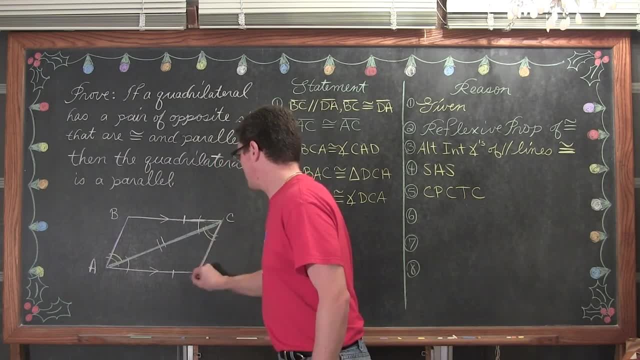 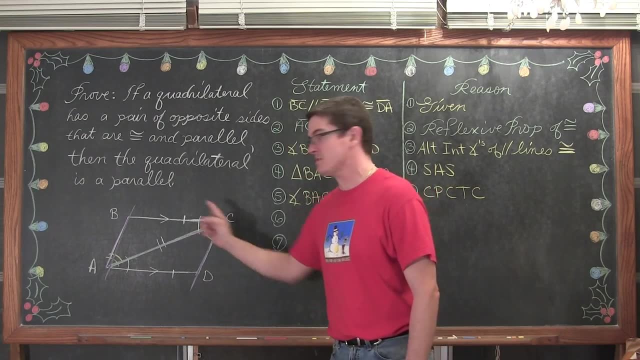 Again, when you have that zigzag shape from two lines being cut by a transversal, when those- Let's see, When those alternate interior angles are congruent, then those lines are parallel. It is the exact- Well, it is the converse of what I used up here in line three. 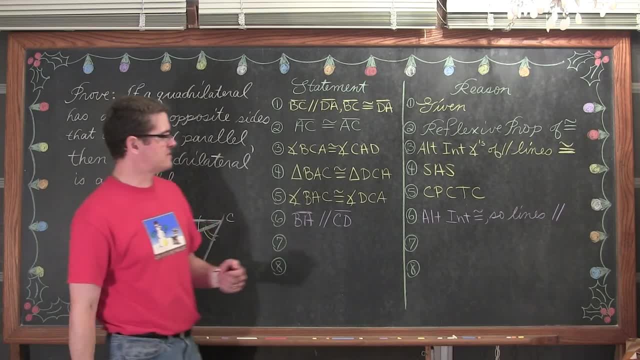 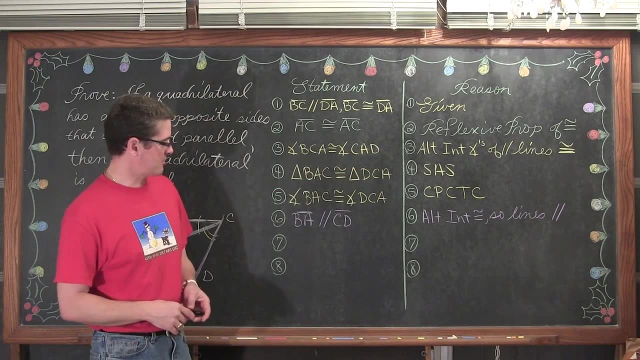 Ok, when you are abbreviating things it is kind of hard to fit this in. so I just said: alternate interior angles are congruent, so my lines are parallel. That is the converse, again, of reason number three. Now I put eight lines down here for my proof, but I am actually not going to need that because 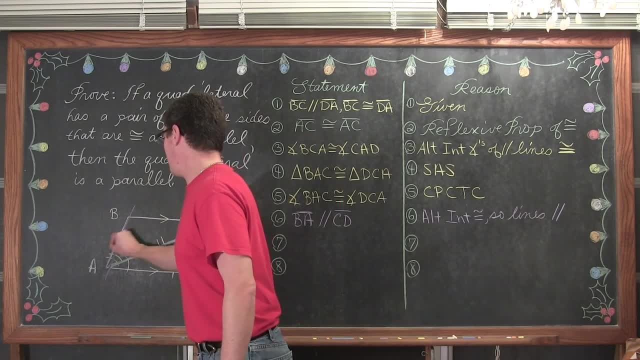 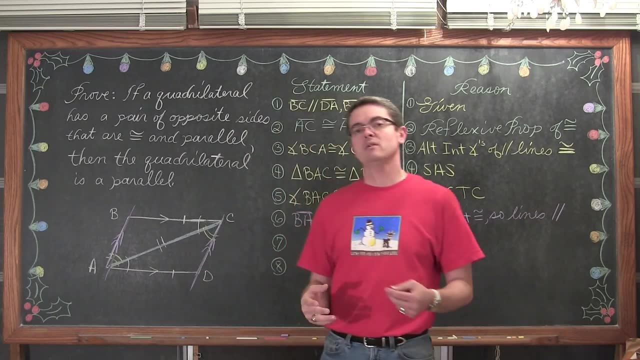 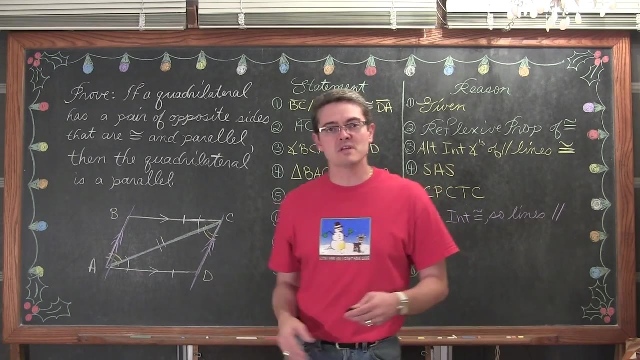 now I have stated that BA is parallel to CD. Ok, And I have a four-sided figure where two pairs of sides are parallel and thus, by definition, this is a parallelogram and my proof is done. So let me just kind of fill in this one last line. 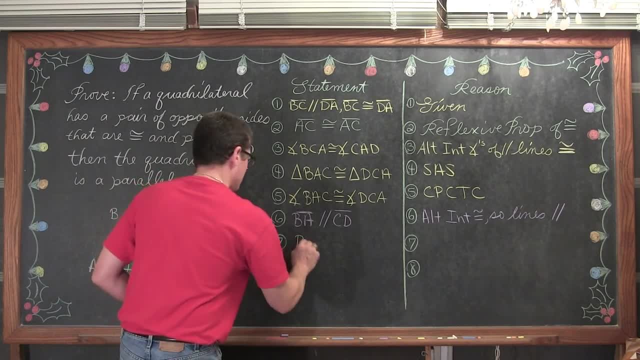 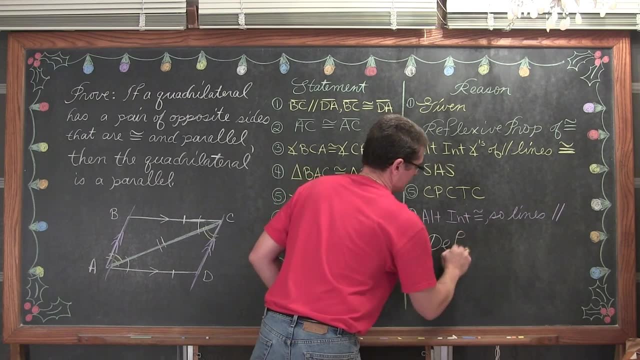 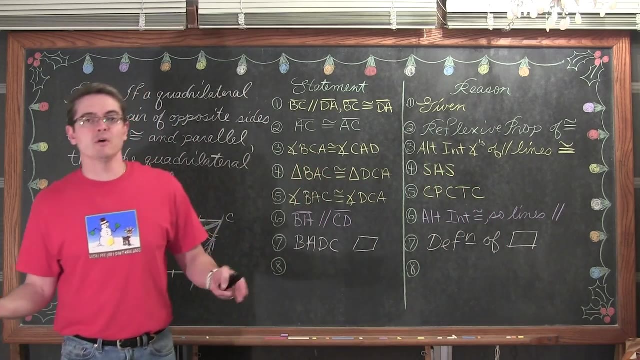 So I will just keep talking and write. We have BADC is a parallelogram due to definition of what a parallelogram is. Ok, That is correct. That is correct. Ok, That is correct. Ok. Now I know where that parallelogram is and that is going to be my proof. So I am Mr Tarrou BAM: Go Do Your Homework. 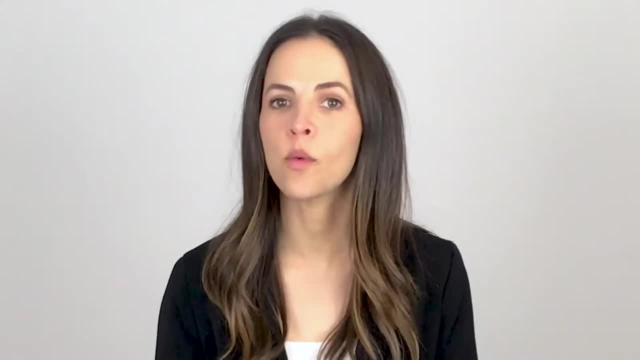 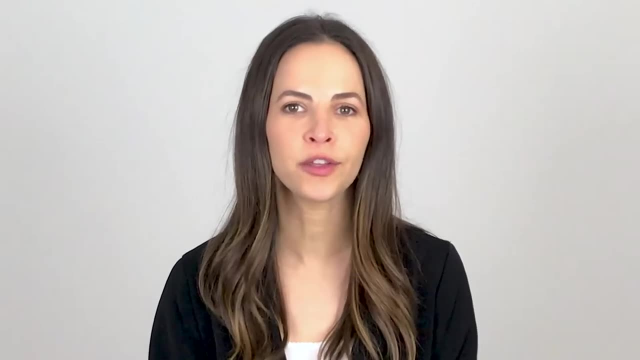 Ideally, you'd file your taxes using a W-2, but if you're watching this, chances are your employer didn't provide a W-2 form or you lost your old document. No worries, you can still file your taxes in a few quick steps. Keep watching to learn how you can file taxes using your last pay stub instead. 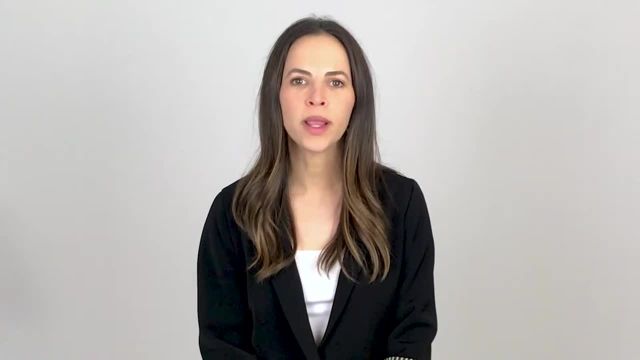 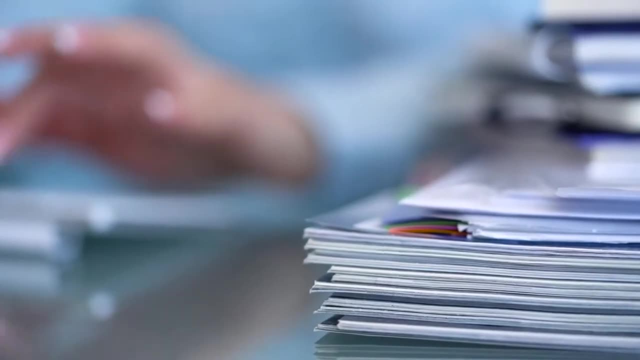 of a W-2. Filing online. For those wondering, can you file taxes with your last pay stub? The answer is yes, but the best way to do so is online. It is possible to use a pay stub to file taxes in. 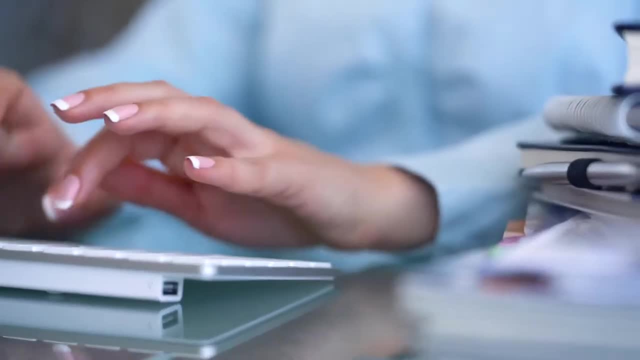 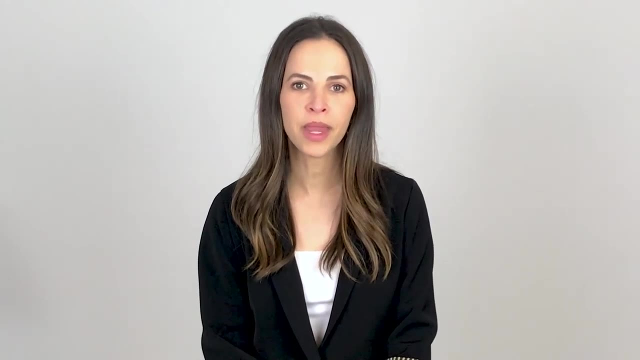 the traditional way, but you'll need to notify the IRS that you're doing so and fill out a 4852 form. You should note that there are some exceptions, though, so filing online may not be your best bet. According to the IRS, the maximum gross income threshold for those wishing to e-file- for free. with the IRS. free file service is currently $57,000.. Similar restrictions apply for those under the age of 16, as well as residents in Guam, the US Virgin Islands, the Commonwealth of the Northern Mariana Islands and the United States. For those under the age of 16, as well as. 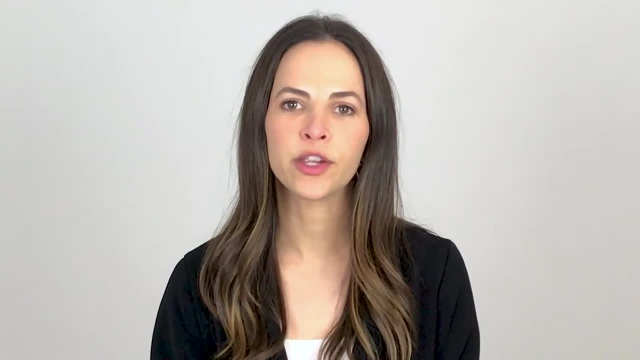 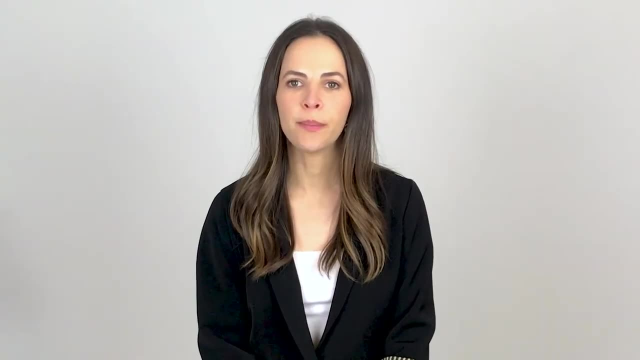 residents in Guam, the US Virgin Islands, the US Virgin Islands and the United States. You can still prepare your return online, but you will have to print and mail it. if any of the above applies to you, How to file: Essentially, a pay stub will be able to provide most, if not all. 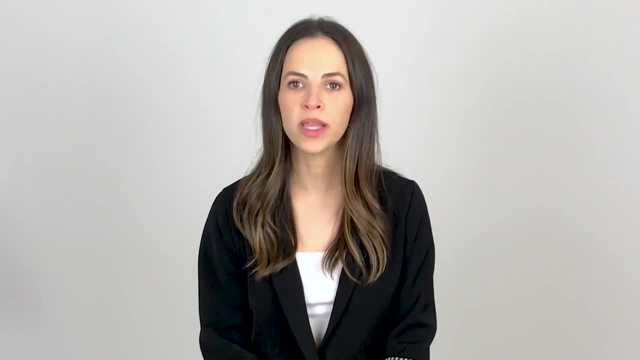 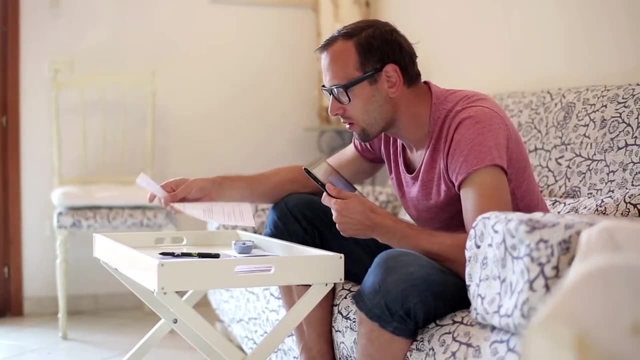 of the information you need to file your taxes that you would normally get from a W-2.. Your pay stub will, of course, have your monthly or biweekly income on it, which is the most important piece of information the IRS needs. It will also list any tax deductions that come out of your paycheck. 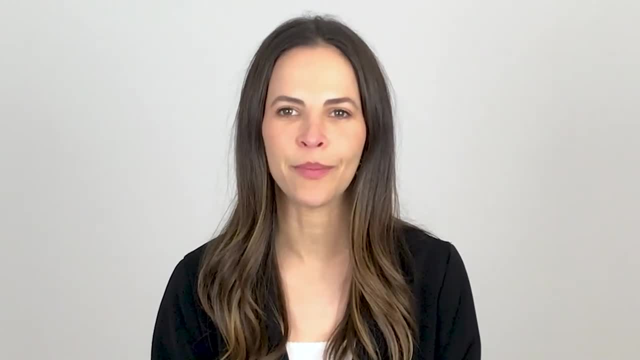 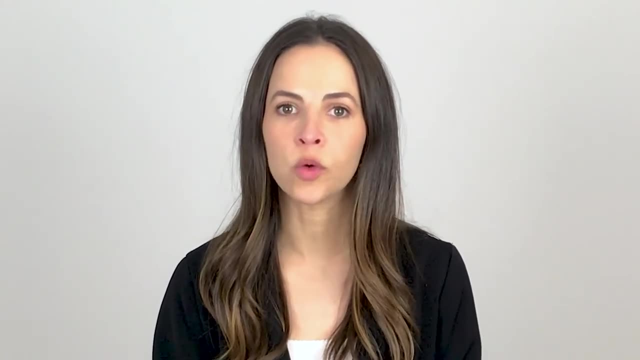 Filing your taxes and filing them accurately isn't always the same thing. To make sure you have calculated the right amount and that you aren't paying too much or too little, you'll need a tax calculator, which you can find online. Add in your year-to-date taxable income alongside any leftover taxable income. 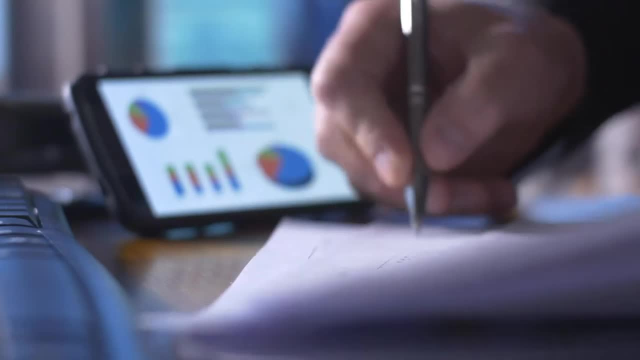 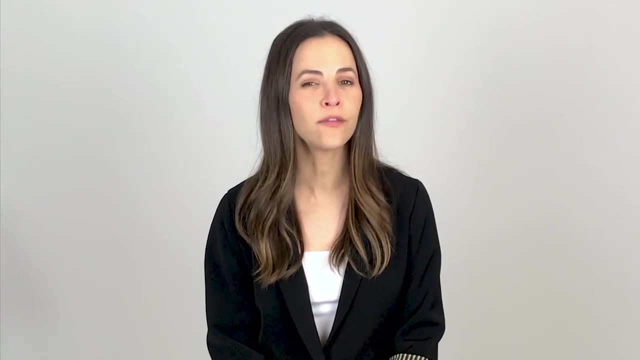 that is not in the pay stub you're using to file your taxes. You'll also want to include any relevant expenses, like dependents. It's a good idea to run this info through the calculator several times to make sure you're getting an accurate result.